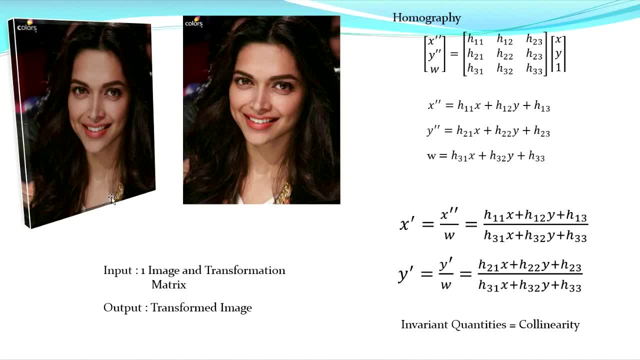 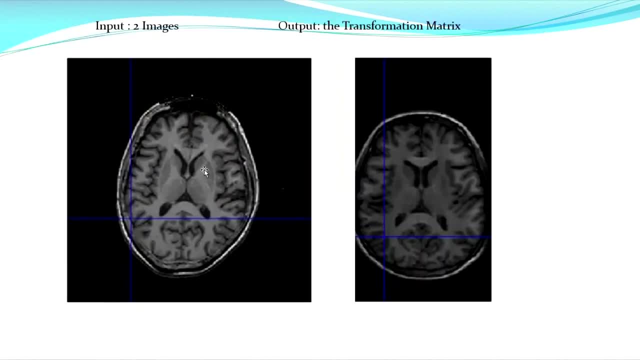 we want to perform on it and we will perform and do this kind of a thing. So this is what we have seen till now. Now what happens in registration is now we are given with two images. So my input is two image and what is the output? So the output should be the transformation matrix. So these two images I have. Now you tell me the transformation matrix by which I can convert one image to. 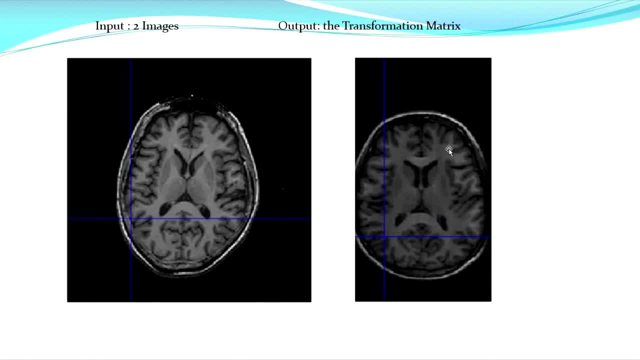 other. So that is my task. So this is what we call by registration of an image or image registration. So one of the most practical examples of image registration or application, practical application of image registration, is in MRI. So these are MRI image of two different subjects, So brain scans of two different subjects, And we want to make some study on this brain scan. 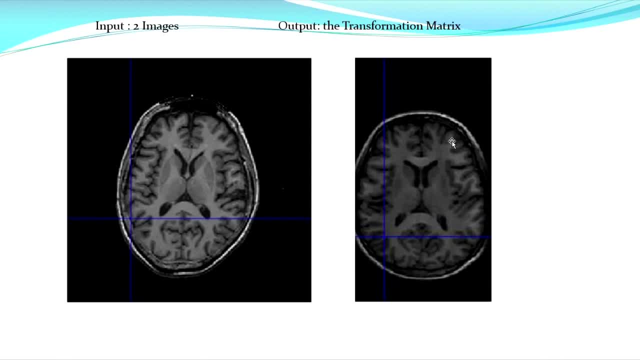 So, in order to do that, it is very important to first align both of these images So that so it is like putting one brain on the other and and it much, as much, as much it can. So that is how to Вut what we have to do. 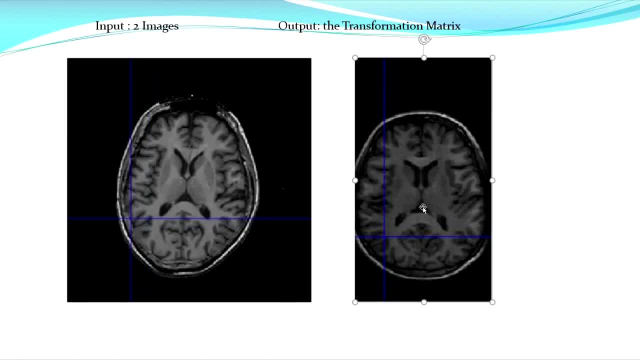 So let us see how can we do this, So, So, manually, if suppose I would tell you if you want to basically do that, So what do you? this, do this, So what do I have to do? Myじゃあ, we would do is we would put this over here and we would see how much is the 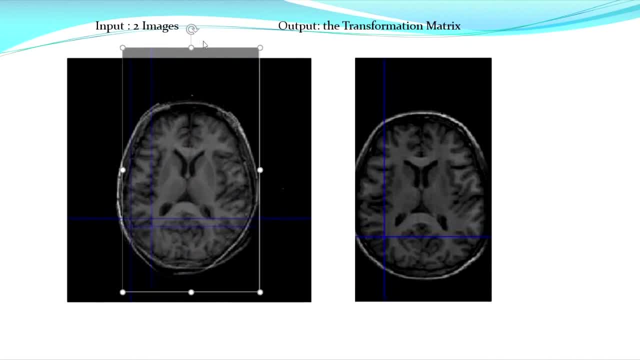 match, so we think this is okay, kind of a thing. but then we see that if suppose I rotate this a little bit, so I'm rotating it and so I think this is not that much matched. let me low rotate it little bit. yes, I guess this is quite ok, kind of a. 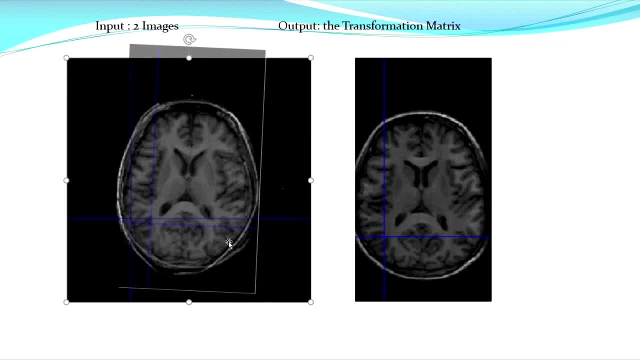 fit. so this is something that we can do. so you saw that I took this image, I rotated it- it's in some particular angle, I don't know the angle- and then I did some translation so that I can get these boundaries match to each other the total number here in, because the second column is the number of columns and the 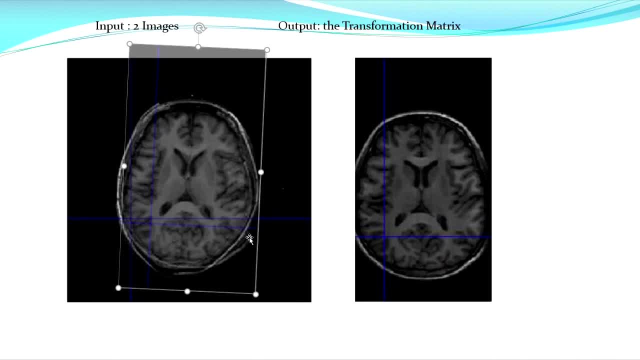 total number here in. because the total number here in, because the total number. total match will not be possible because they are of different subjects. so the head size may be different, right, but we want the maximum match. so after this, only I can perform a particular study as to which part of the brain is involved in a particular task or something else. so 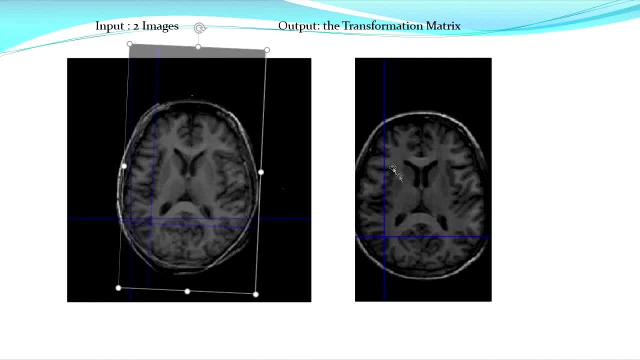 this. so please understand the problem over here. I have been given with two images and I want to find out what transformation matrix will give me this kind of a transformation. so I am transforming this image. so here you can see that I have transformed this image to this thing over here such that now I can work with both the images, which are aligned. 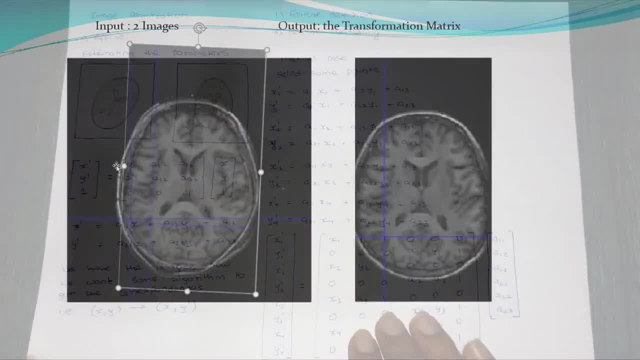 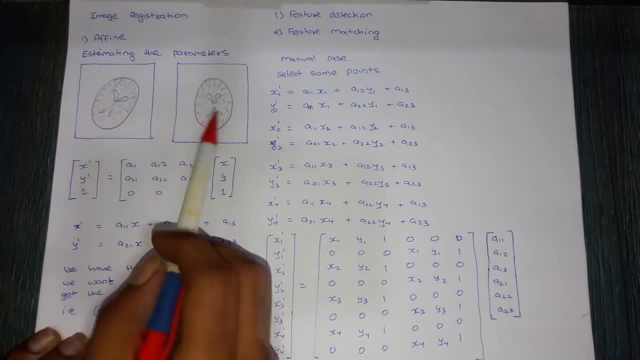 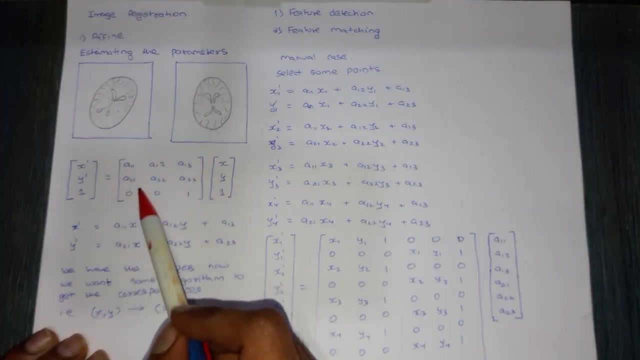 so this is what is known as registration of image. so let us see how can we do registration. so we saw that we have M Say, these two are the MRI images and I have to find out this parameter matrix. So let's start with affine transform. 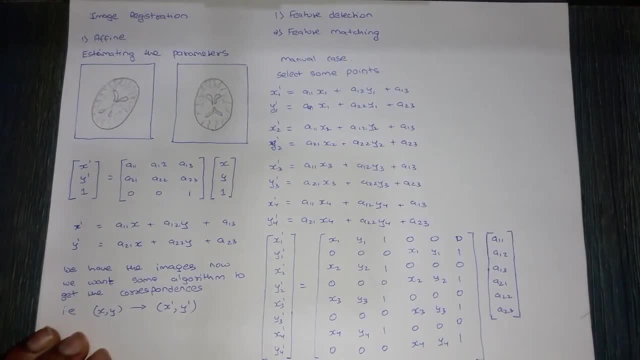 So suppose that I am just assuming that the transformation between these two images is just affine. So we are not including the homography case Now. we will see that case later. So this, this six numbers, are what I have to determine or estimate. So I have to estimate these six numbers. 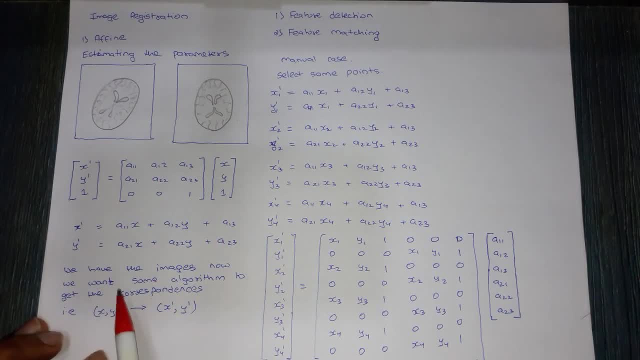 I have been given with two images, So if suppose I make it in equation form, so they will look something like this: So I have, X dash is equal to A11X1 plus A12Y plus A131.. So this is what I have. Similarly, Y dash. I can, I can make these equations. 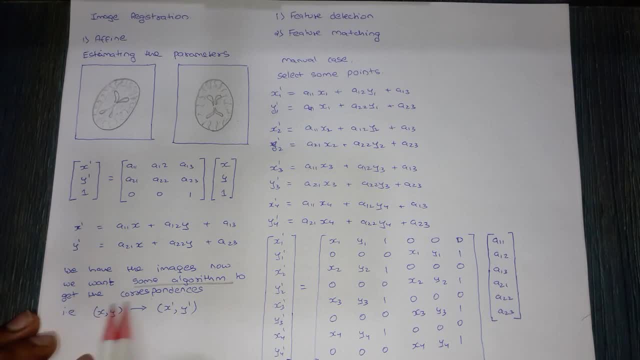 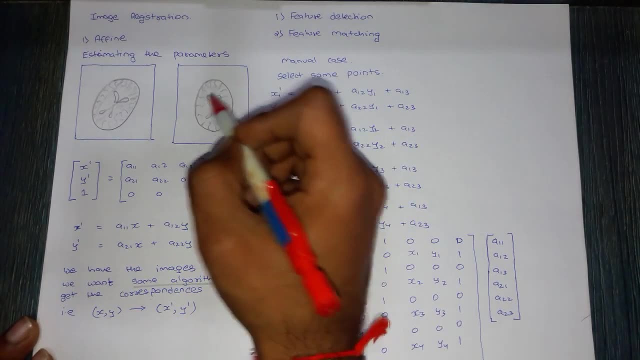 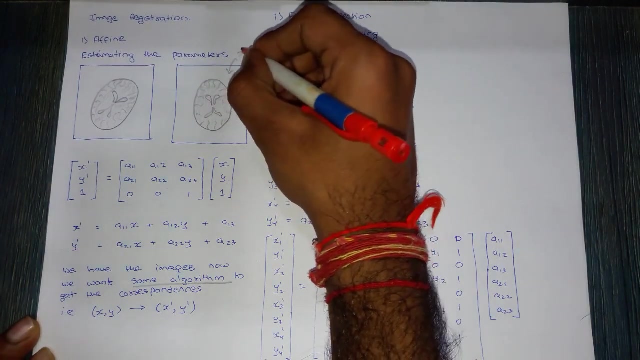 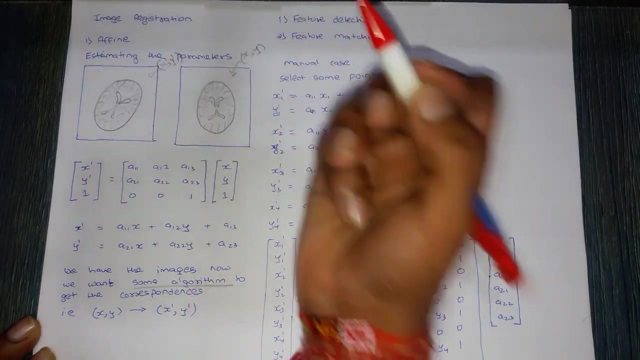 So we need some algorithm to get the correspondence. Now, what is correspondence? I should know if suppose there is one, if this is the X comma Y. So let me take that every pixel in this image will be denoted by X, Y and every pixel in this image will be denoted by X, dash, Y, dash. 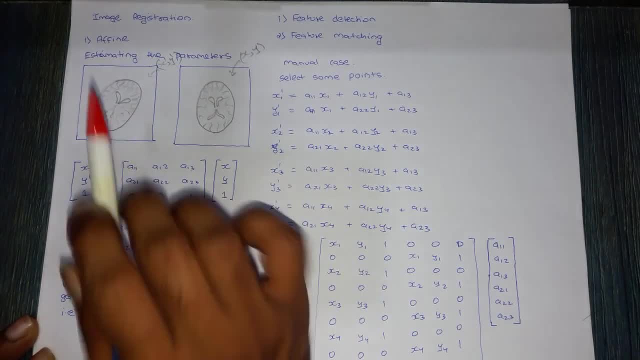 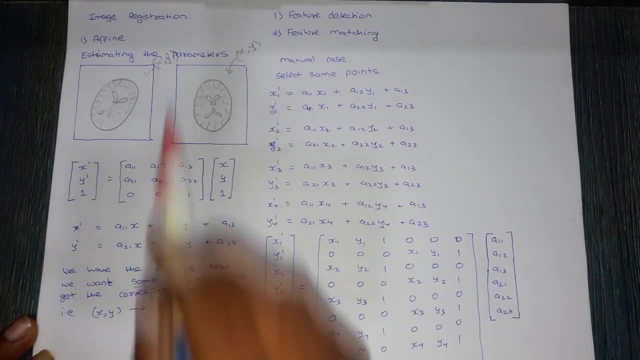 So I want to transform this image so that I can get this image. This is my goal, right? So let me do this: X, Y, and this is X, dash, Y, And this is X, dash, Y, dash. So now what I need is: I will need to select some points. 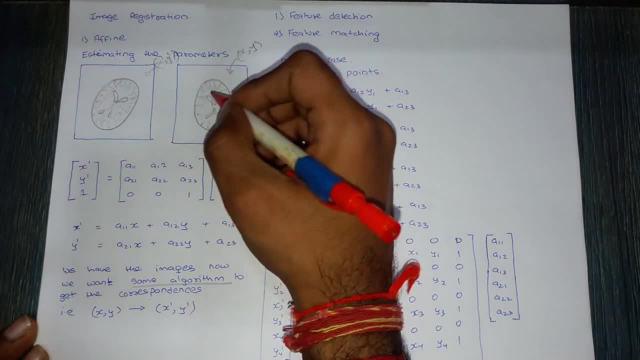 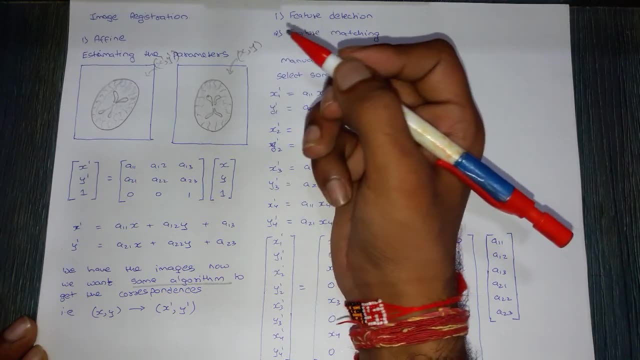 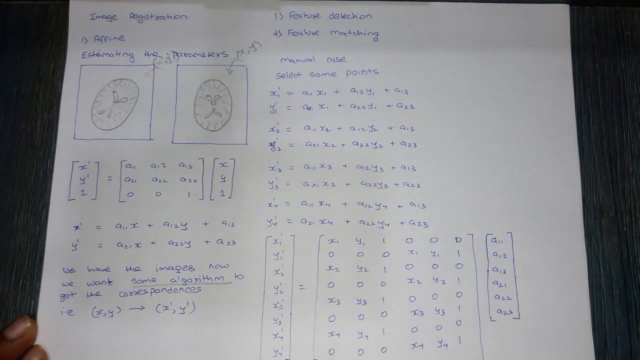 So that is as follows: So suppose. so what I want to say is I want the algorithm to know if there is this point over here. If suppose there is this point over here, then this corresponds to this point over here. So please understand. 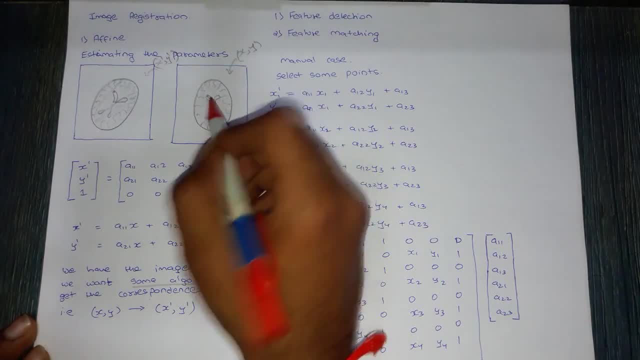 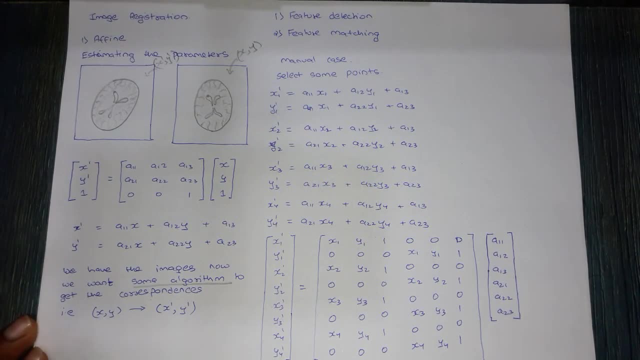 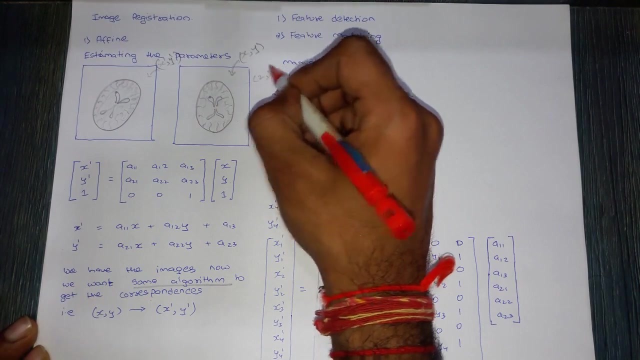 So I want to tell him that How has the points transformed? So this point has transformed over here. So this is what is correspondence. So say, this pixel location, This over here is some say 2 comma 3. This is the pixel location over here. 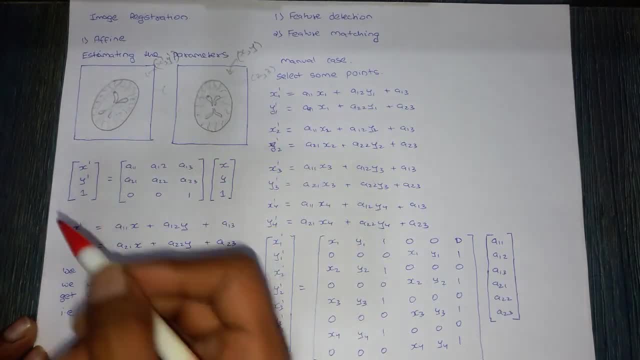 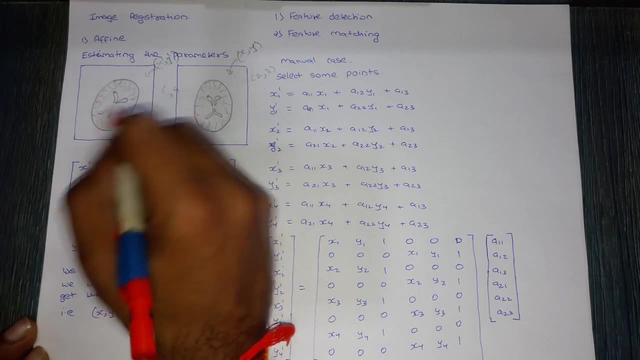 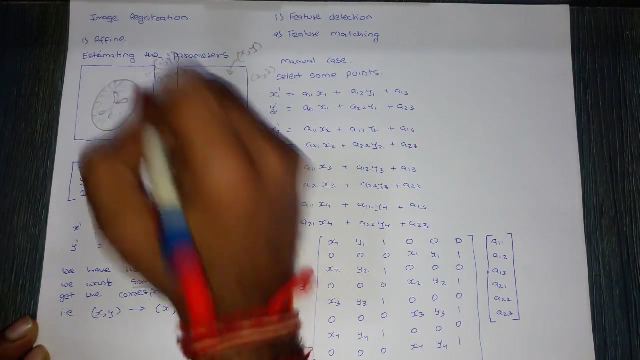 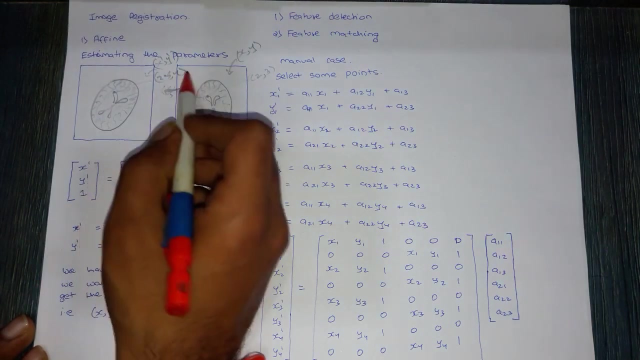 And this has transformed, to say some, This has gone a little upright, So let me take it as 4 and this has gone like this 2.5. So suppose it is 2.5 comma 4.. This particular thing, So I will have to say that this 2 comma 3, this point over here, got transformed to 2.5 comma 4.. 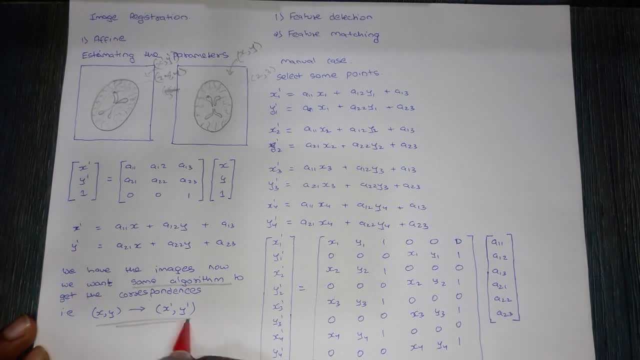 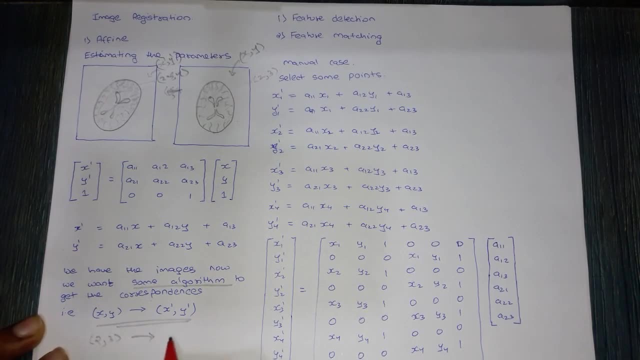 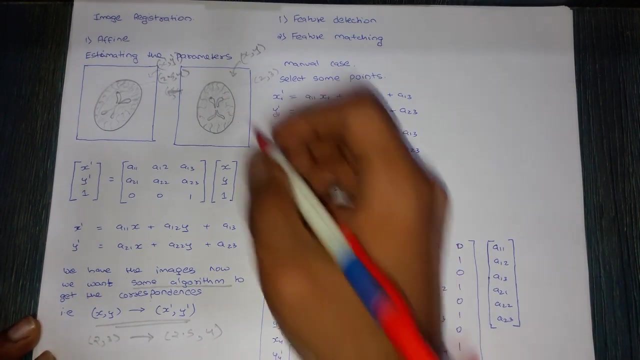 So like this: I will have to have correspondences, So this is what is called as correspondence. So I say 2 comma 3 corresponds to 2 comma 2.5 comma 4.. This is one correspondence That I have. The other correspondence is like this: 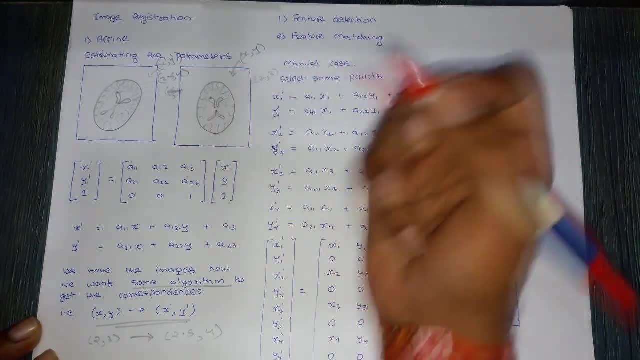 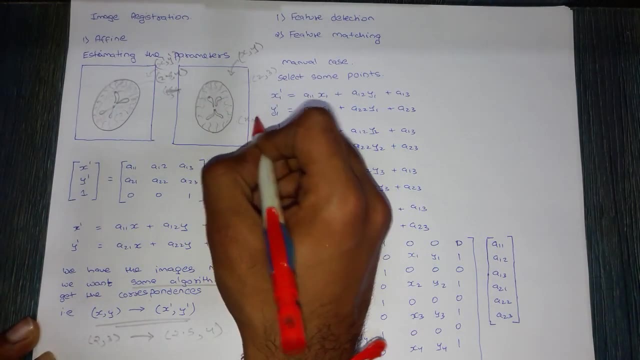 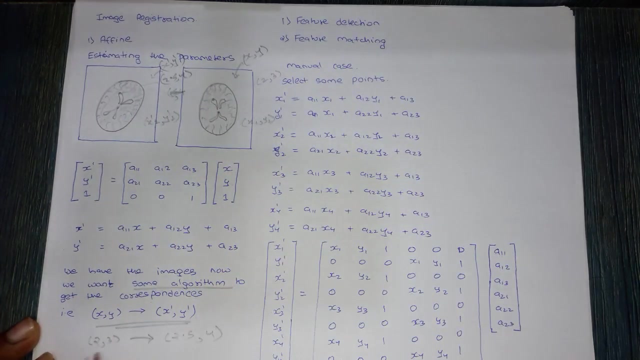 Suppose, if I take this particular point, So this point, I will say maps with this point over here. So this will be my. some other say x2, y2.. And this will be my x dash 2, y dash 2.. So that is what is happening. 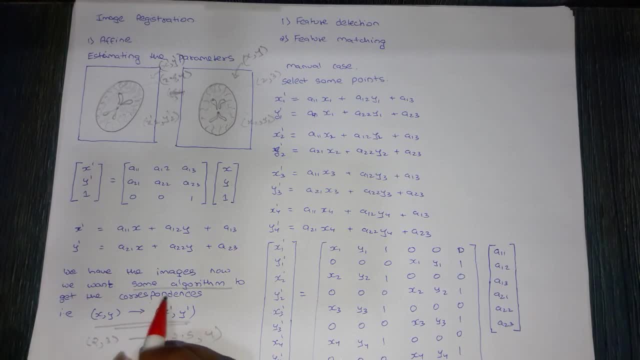 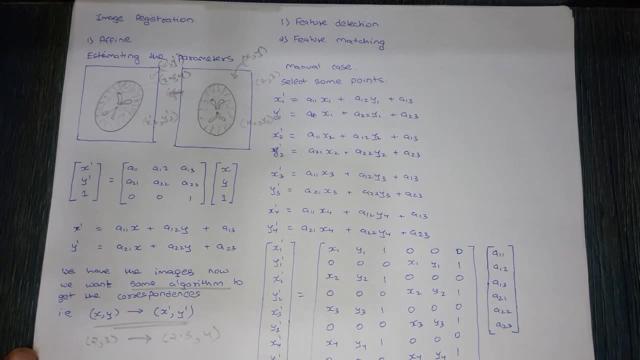 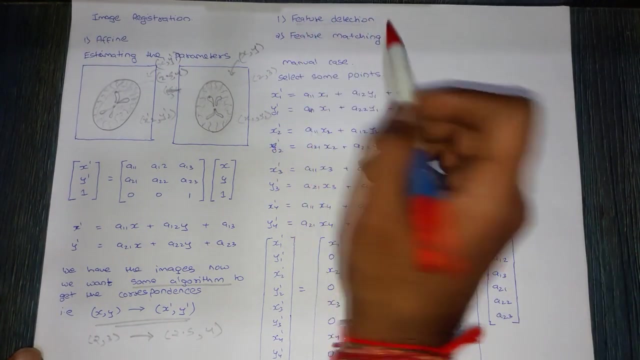 So this is correspondence, So we need some algorithm that can tell me what are these correspondences. So, in order. So for this registration, basically there are two things that we need to know. One is the feature detection, Other is the feature matching. 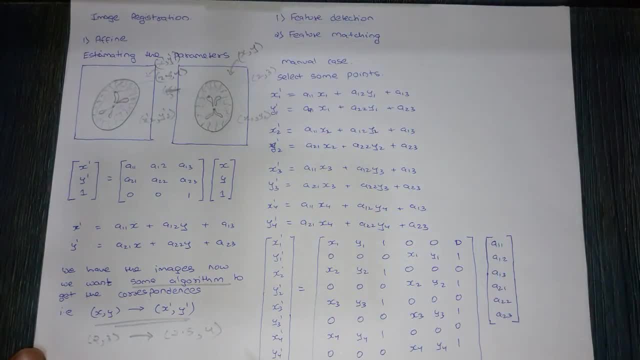 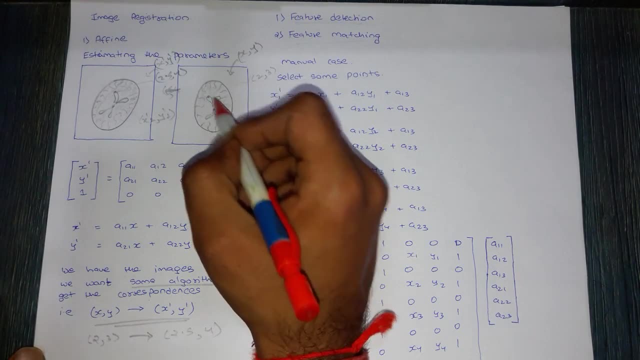 So what is feature detection? Feature detection is it tells you which particular points to map. So now you see that I chose this particular point over here and this point over here. I did not choose an arbitrary point like this over here, Because, if you see, 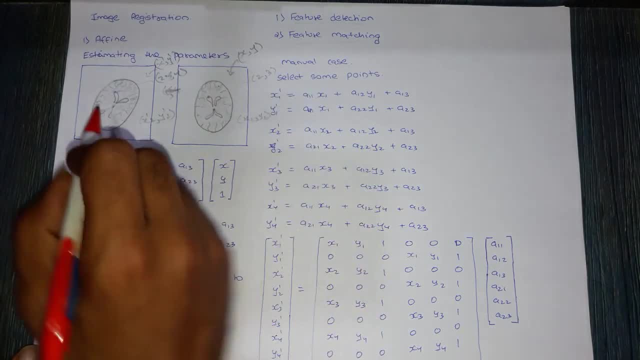 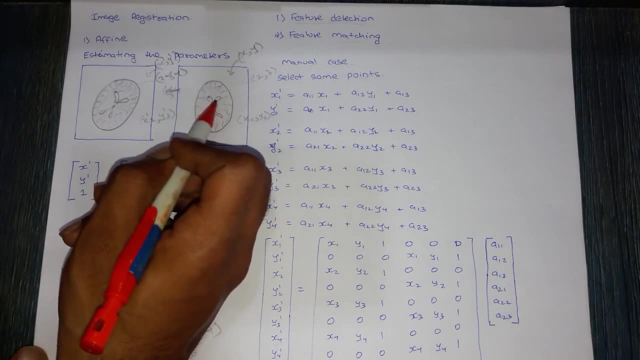 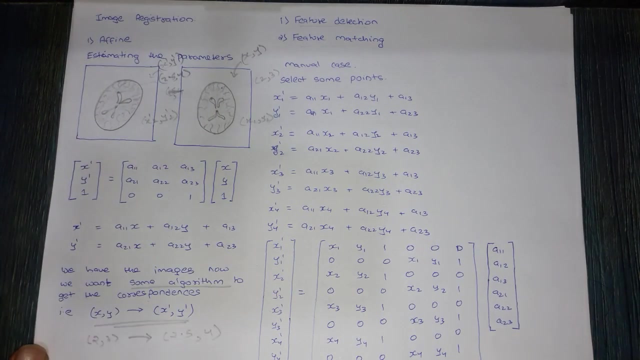 If I choose this point over here, It will be difficult to tell this maps to which point over here. So this is quite difficult, This is very easy. So if I tell over this point over here, I exactly know this point should correspond to this point over here. 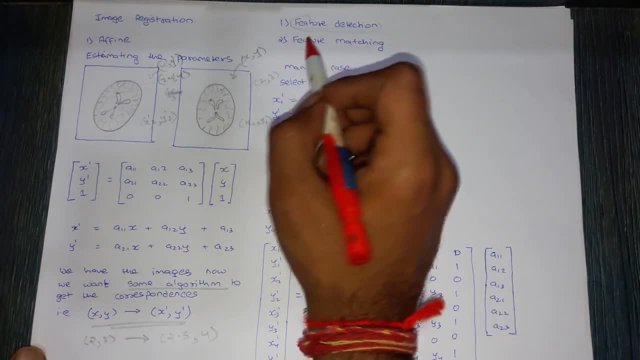 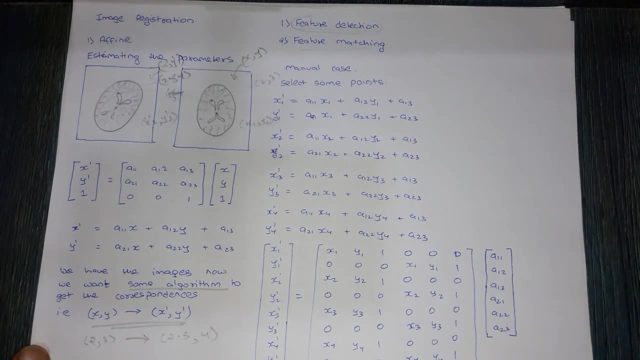 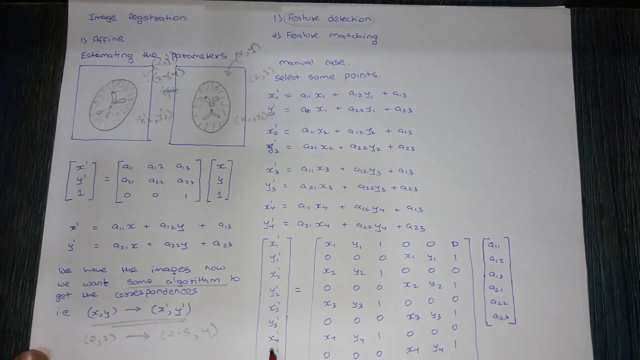 Right. So that is told by feature detection. So the feature detection will tell you which points are important. That will give you more information about the transform. Other is the feature matching. The feature matching is basically the transformation that we do. So now let us here consider a manual case. 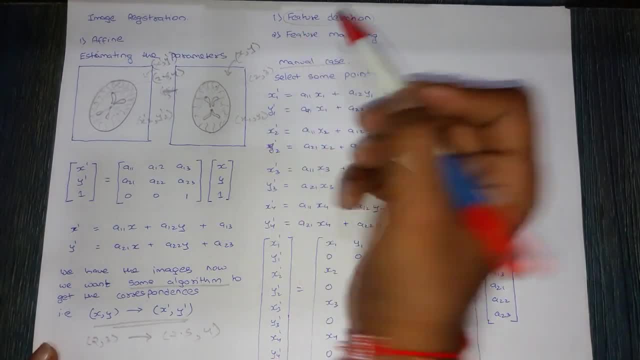 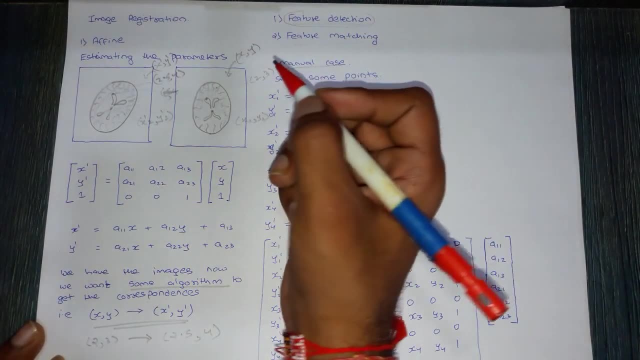 So in the manual case, what we are going to do is We are going to select the points that we want to transform. So, as here, I selected this point And corresponding to this point is this point. So this is my input sort of point. 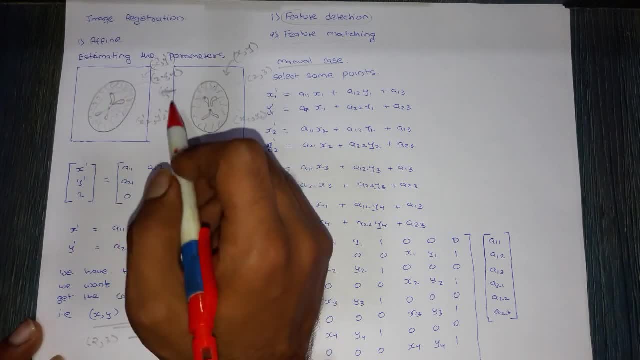 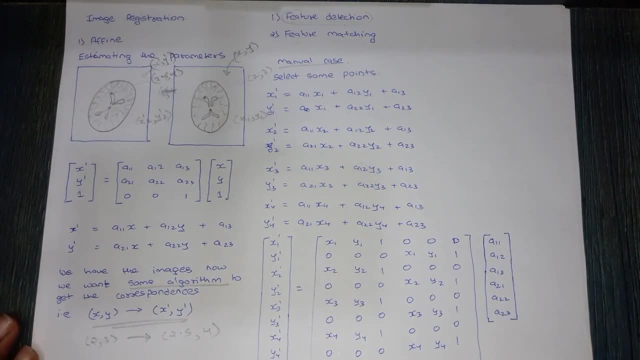 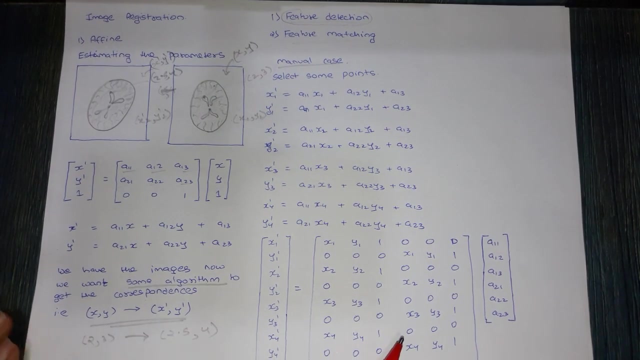 And I want this point to get transformed to this. So that is the first point. So, like this, I will select some number of points. So why am I doing this? I have six numbers to calculate, I have six parameters. Is what we can say. 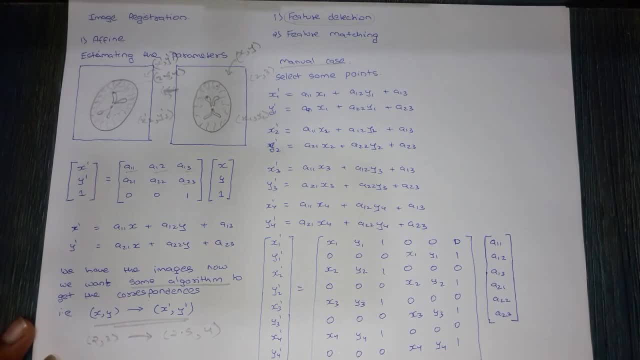 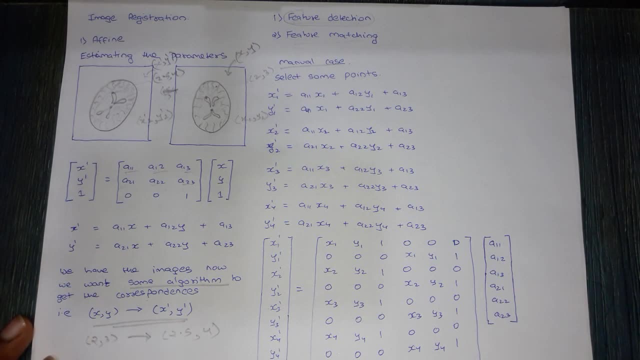 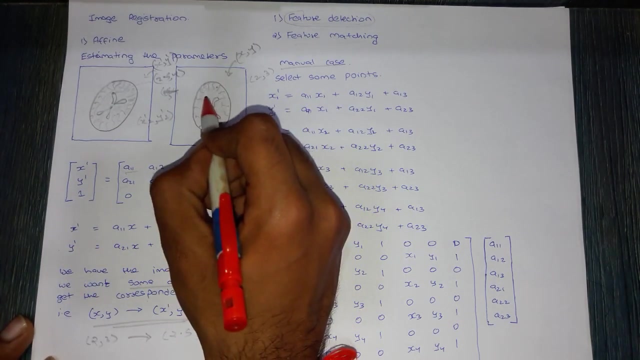 So we know by basic linear algebra That if there are six unknowns We need six equations. So that is what we need. So you can see that one particular point Say: if over here, as I chose, two comma three And its corresponding two point five comma four. 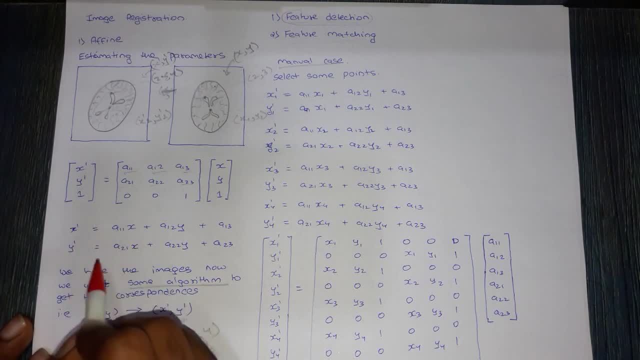 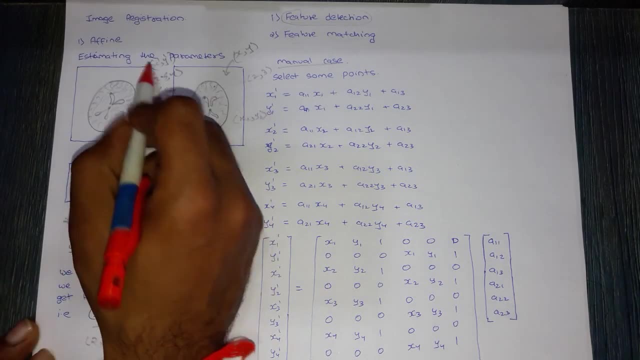 So here, if I put that points in this equation, So this equation, So I will get something like this: So this x dash over here is two point five. So two point five. This was my x dash. Two point five is equal to. 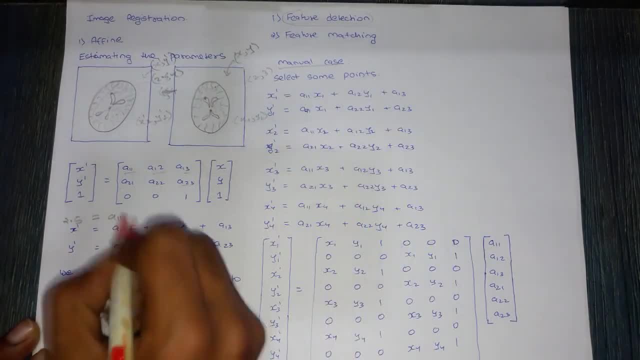 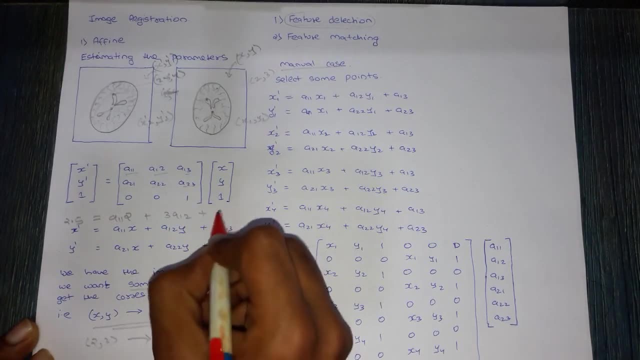 I get a one one into x. X is my two, So two a one one Plus I have y is three, So three a one, two Plus a one three. So like this you can see I got an equation. So similarly I can make for y. 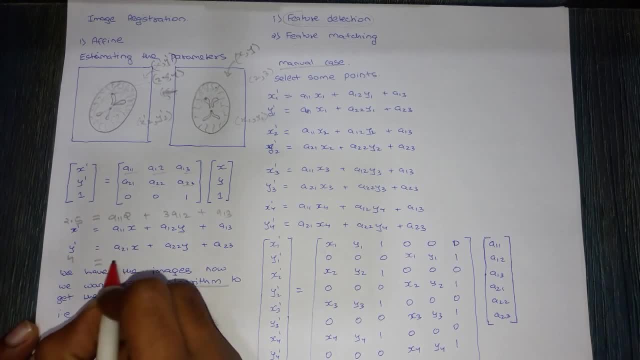 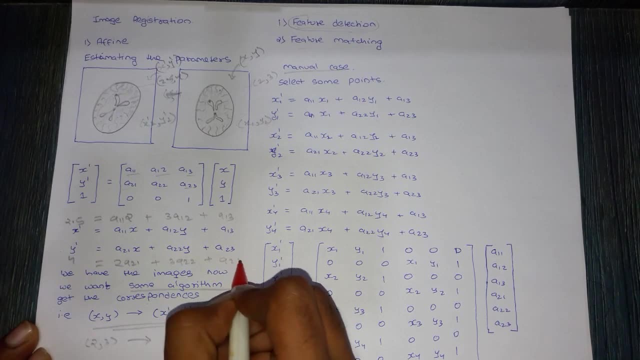 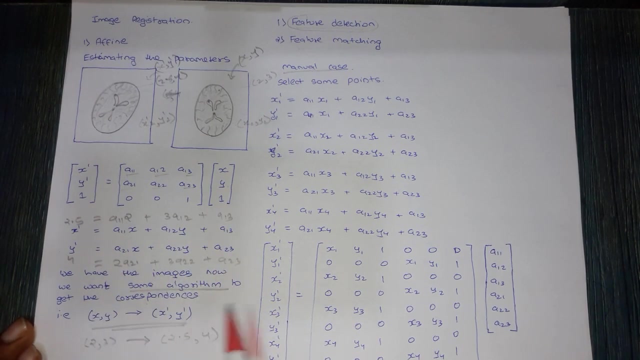 Y dash. So y dash will be. four is equal to Two a two one Plus three a two, two Plus a two three. So like this you can see, I got two equations Of these parameters. So similarly, if suppose, I select some more points. 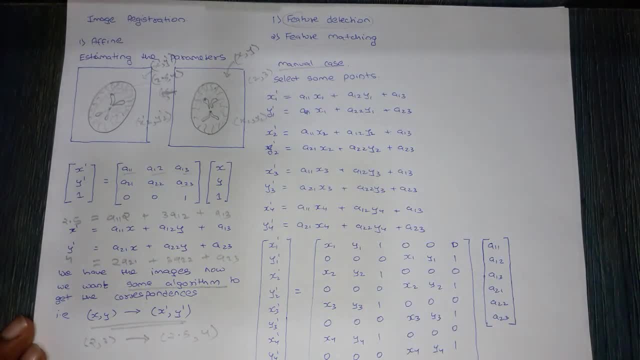 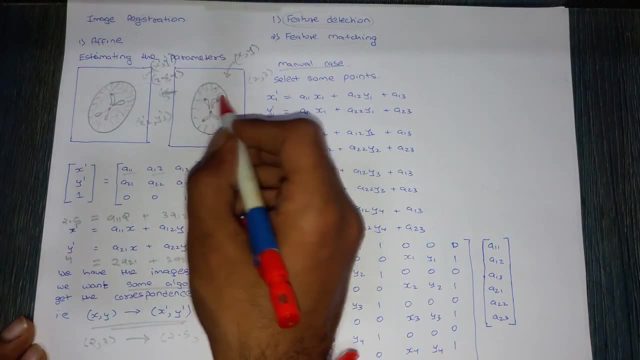 So here, in this case, I have selected four points. So you, I selected this, This and say: this is the other point, This is the other point. So, like this, So this corresponds to this point, This corresponds to this point, This corresponds to this point. 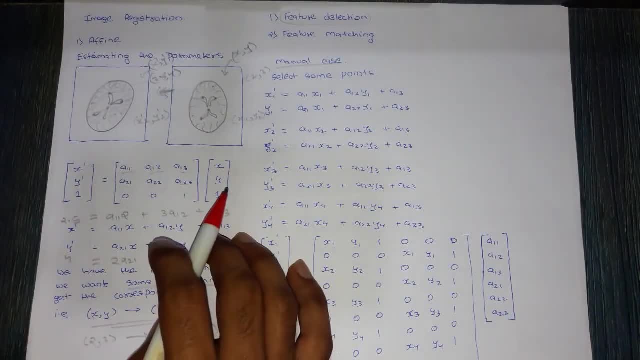 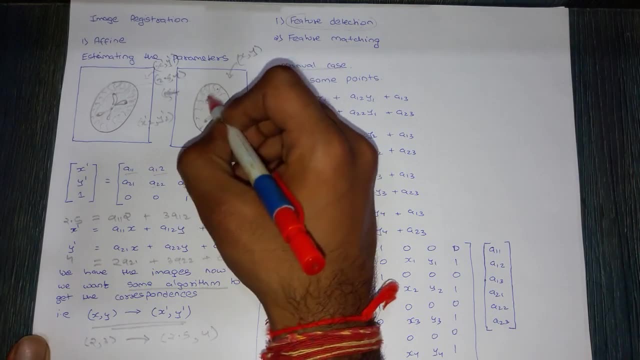 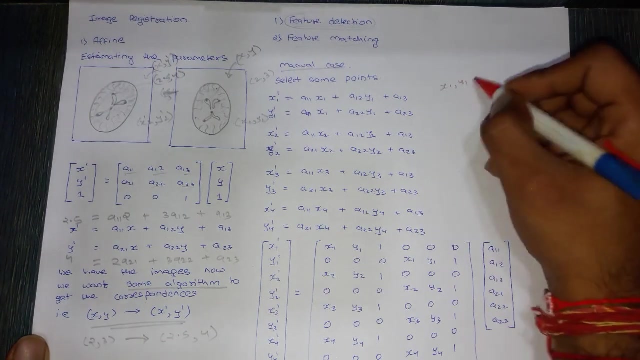 And this corresponds to this point. So, accordingly, I have selected four points And named them as So this point, Let me name this one point. So one point. So one point I have named as X, one, y one, Then its correspondence is x- one dash, y, one dash. 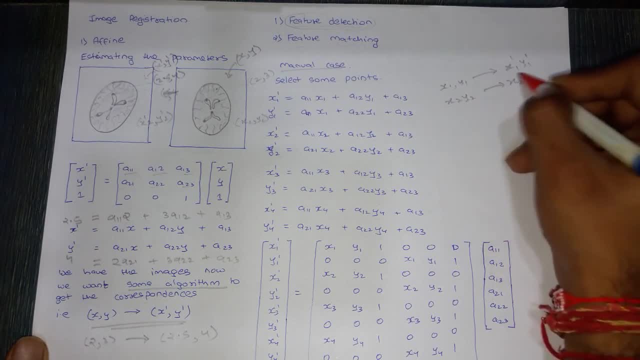 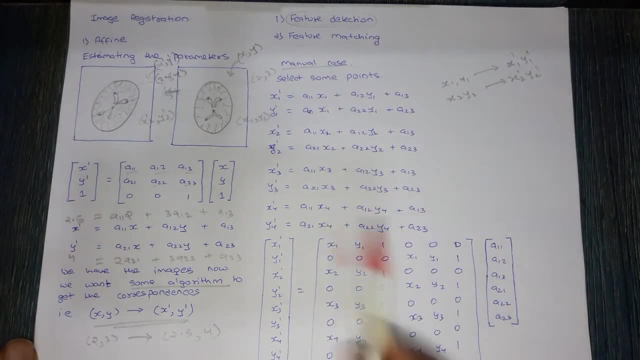 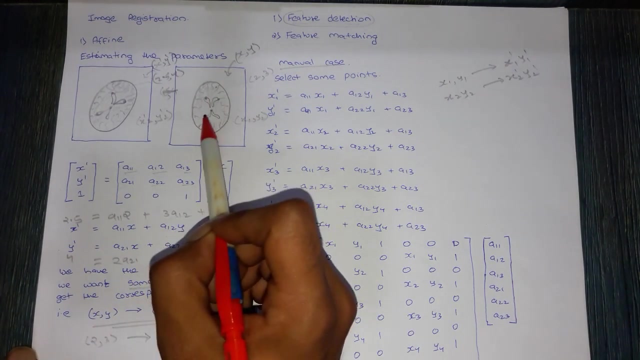 Then x two, y two. Its correspondence is x two dash, y two dash, And the story So like this: I have made four points And accordingly I will get eight equations. So please understand what is happening. I have selected some points manually. 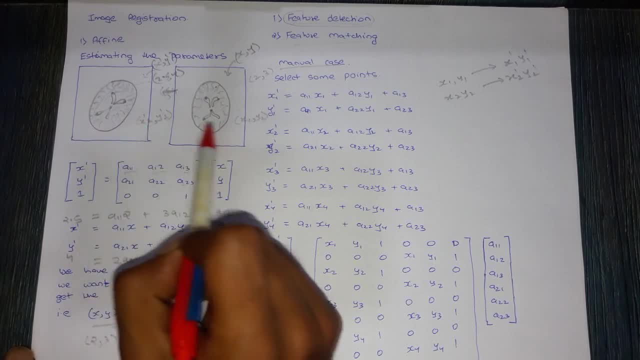 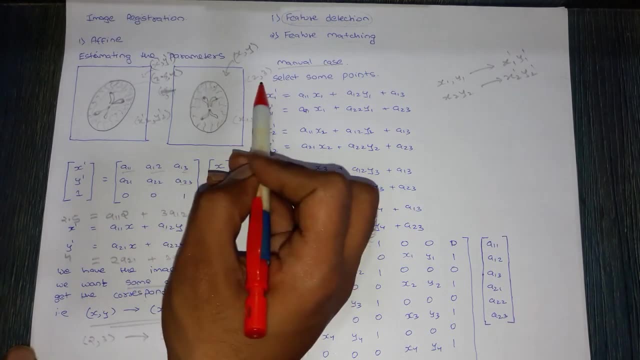 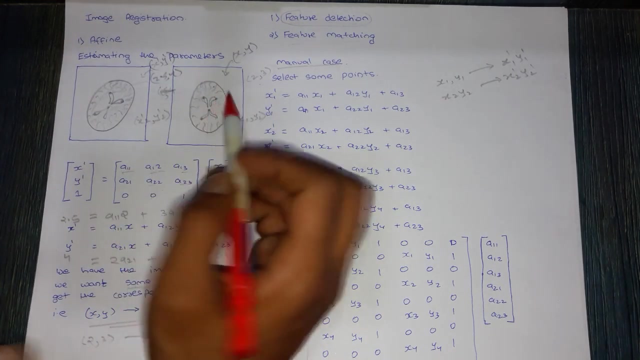 To In both the images So that I can Tell the algorithm or tell the computer That see, this is the point two comma three. I want it to get transformed to two point five comma four. This is the point some Say. let me name this also. 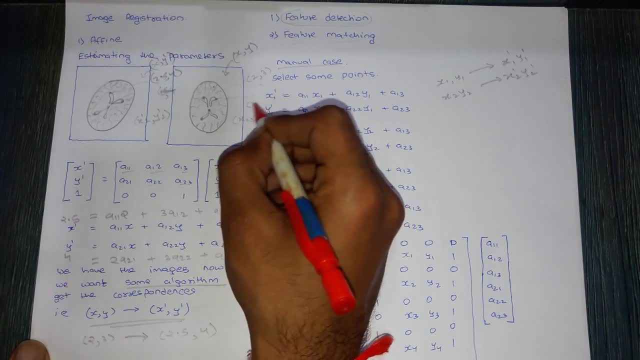 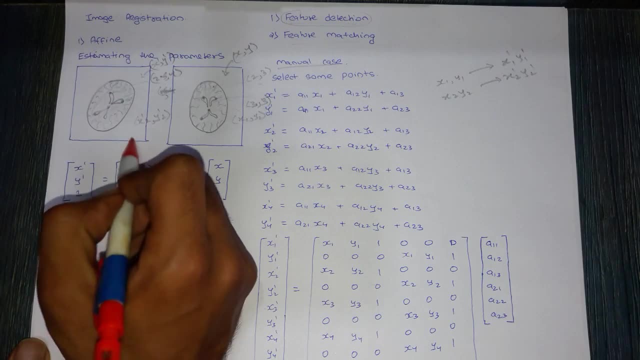 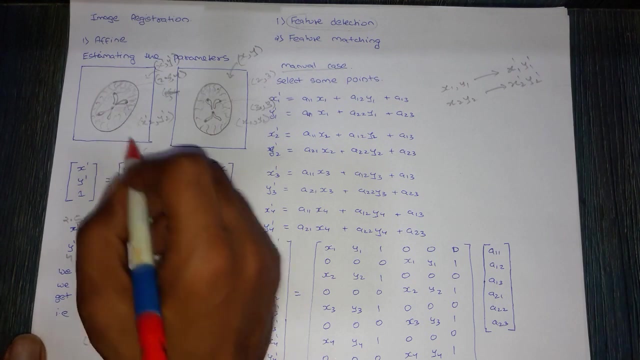 So let this be. So, let this be two comma. This will be three comma Three, suppose. So this three comma three should be mapped with this point over here, Which is some What we say. So let me have this, as This is a little down. 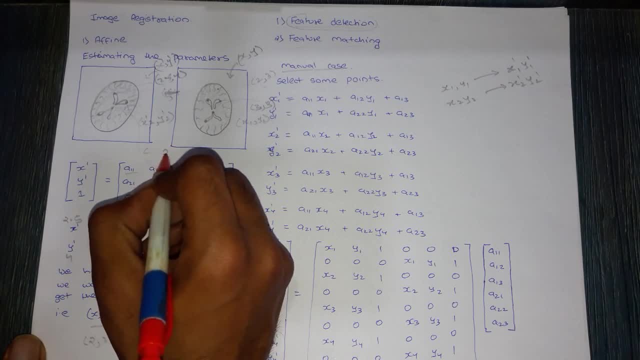 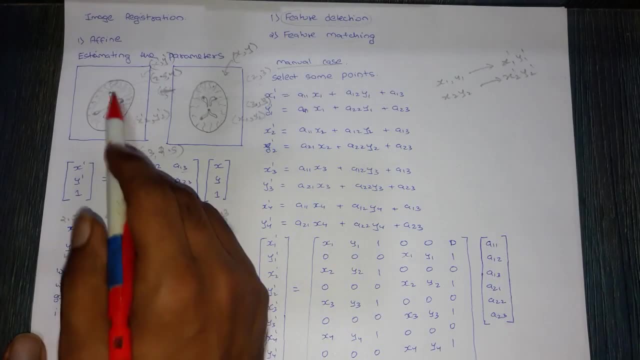 So this will be: Say Four point five, Let this be three, So three comma four point five, something like that. So Please understand what I'm doing. I'm I'm telling the computer. These points should get mapped to this points. 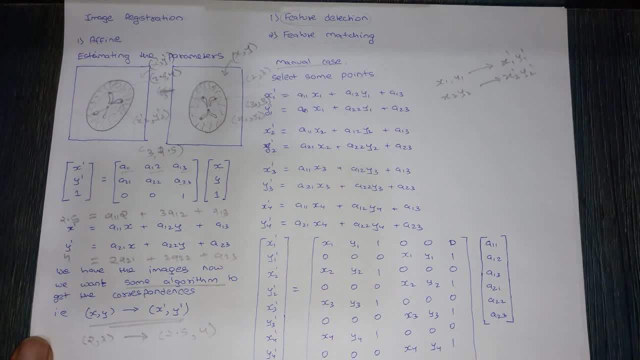 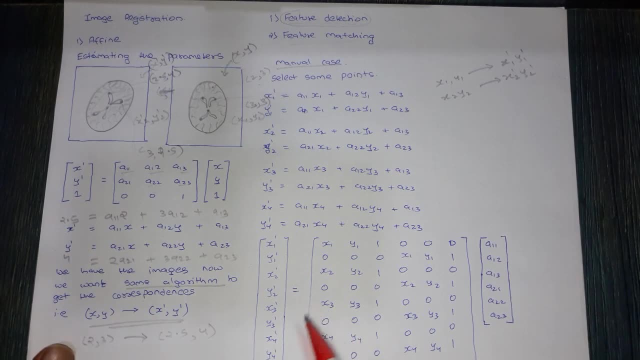 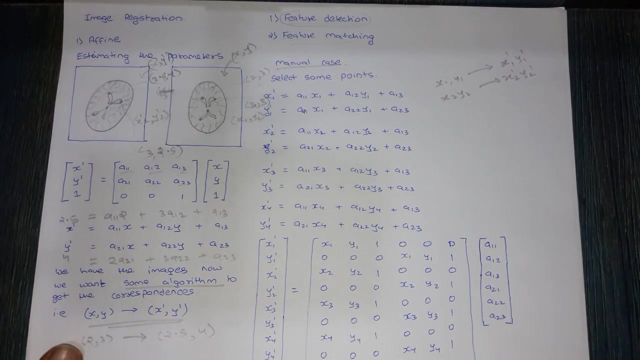 And now I have these equations with, With the information that I have collected over here. Now, what we do is we create a Matrix kind of a thing. So this Matrix, I am creating it just so that I can solve it, So in linear algebra. 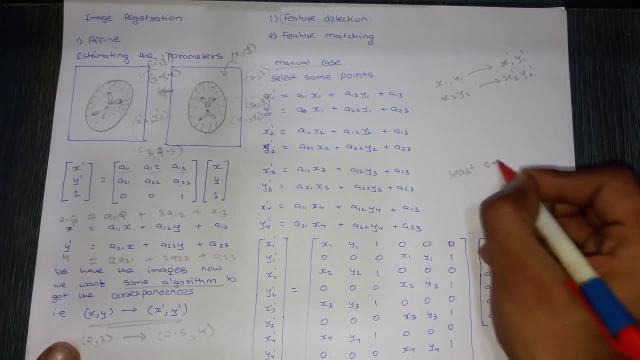 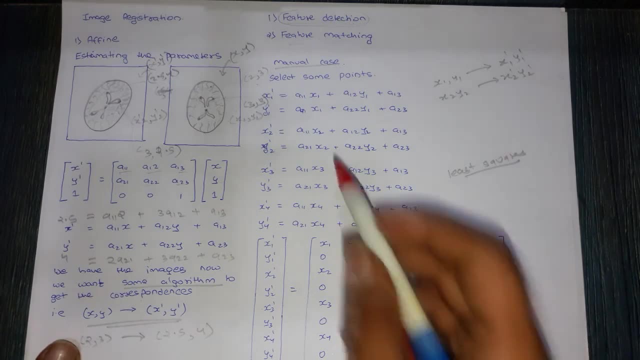 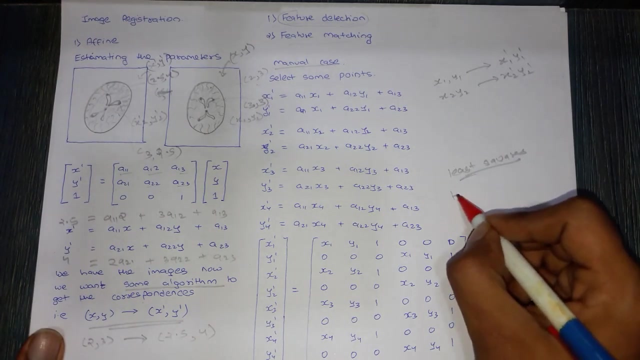 We have least Squares, a method that is least squares. So with using this least squares, We can find out the solution Of these, Even if A one one, a one two And the story So for that. So least squares basically needs this kind of a form. 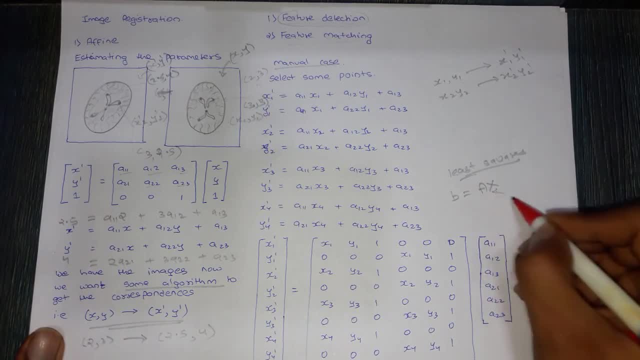 B is equal to AX. So where X is the unknown vector, A is the matrix Which is known And B is also known. So B is known, A is known, X is the unknown. So I am bringing A particular 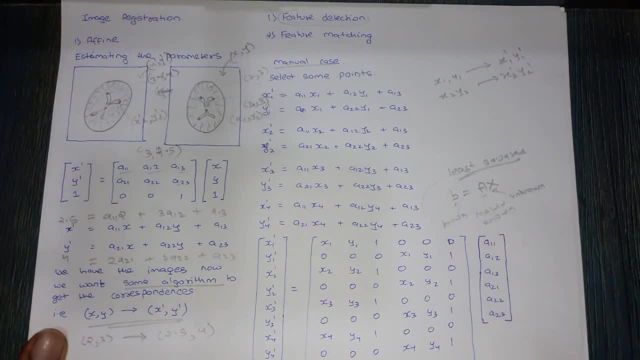 Equation, set of equations into this form. So let us see how. So we know that we These things are unknown: A one, one A one, two A one, three A two, one A two, two A two, three. These parameters are unknown And all other things are known. 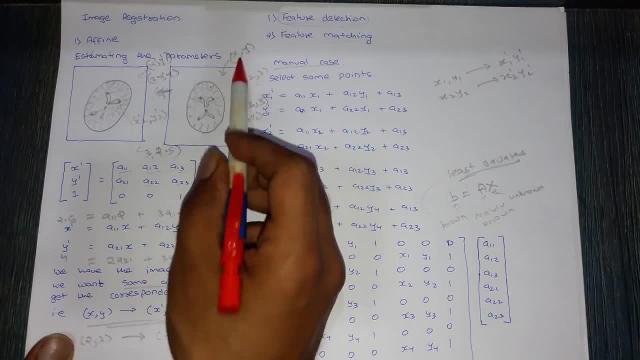 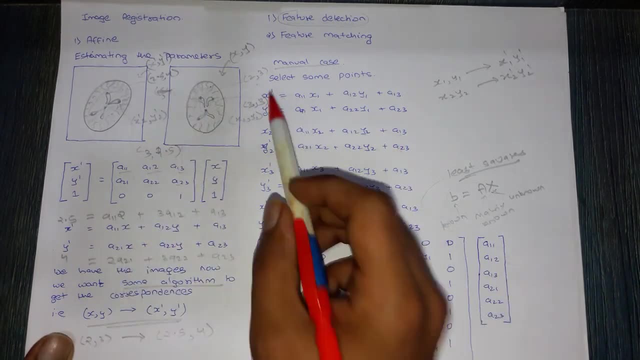 I know X one, Y one, because that is basically my first point. So that first point will be X one, Y one, And correspondingly I will have X one dash, Y one dash. So I know X one dash, Y one dash. I know X one, Y one. 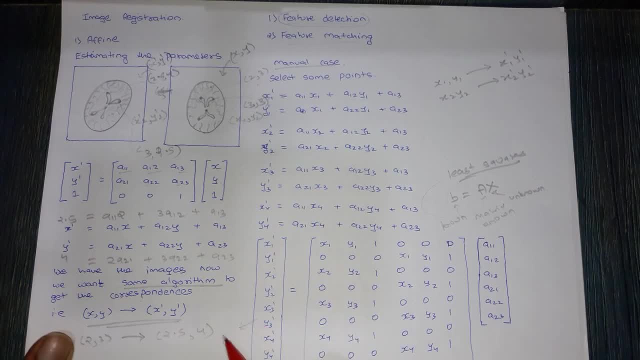 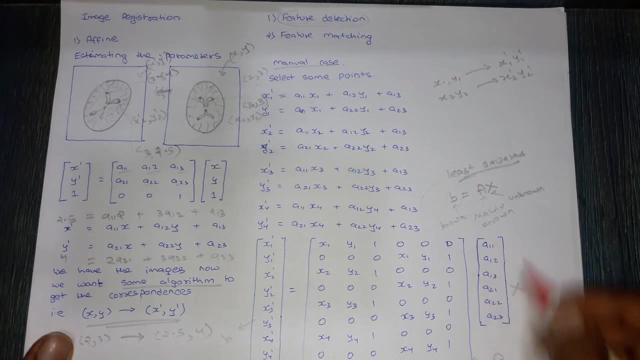 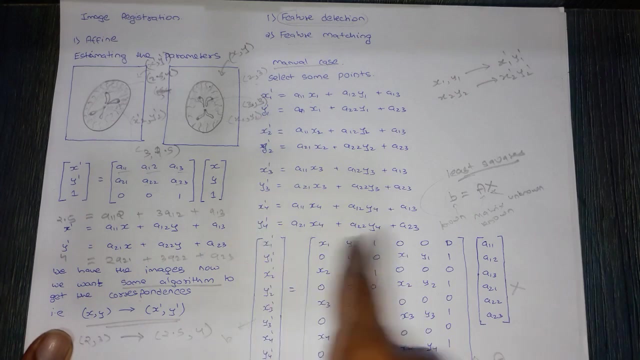 So I know these things. That is my B, for, in least square terminology, This will be my A And this is my X, because this is unknown. So just by doing a little manipulation, You can Make these equations into this matrix form. 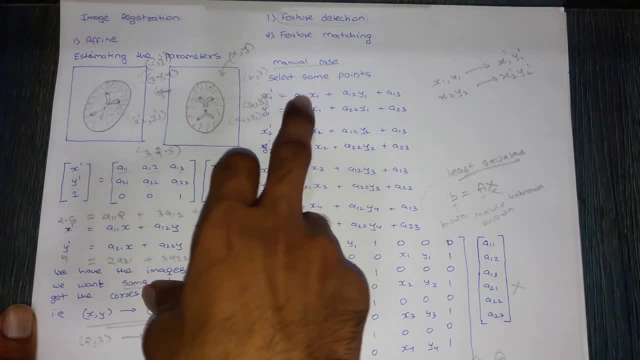 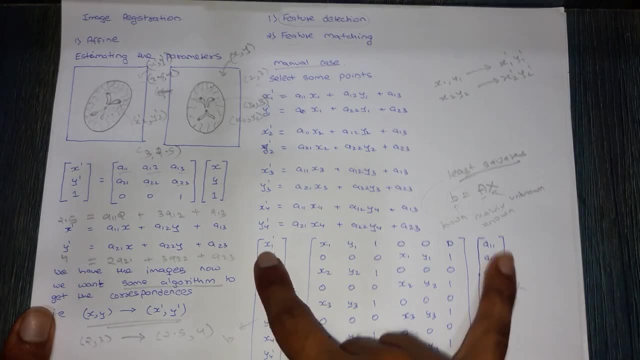 So let us see how I have done this So you can see: X one dash is equal to A one one, X one plus A one two, Y one Plus A one three. So if you see, then in this matrix, So X one dash will be A one one X one, which is what we have. 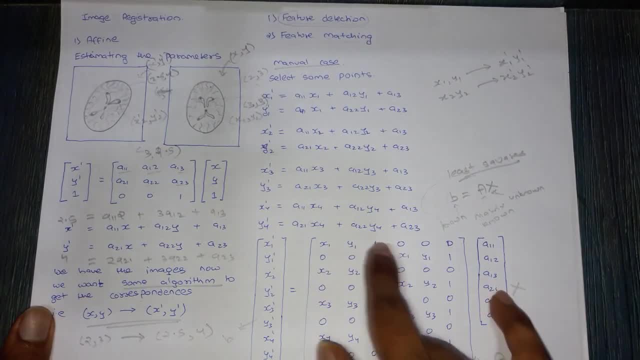 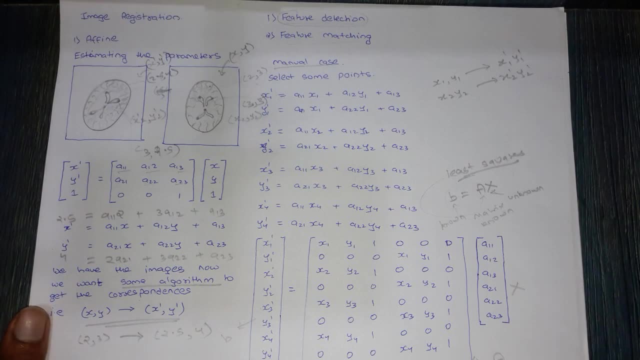 Plus A, one, two, Y one, which is what we have, Plus A, one, three And all zeros. So accordingly, if you work out, you will get this kind of a matrix. So after you have this kind of a matrix, you have this particular form. 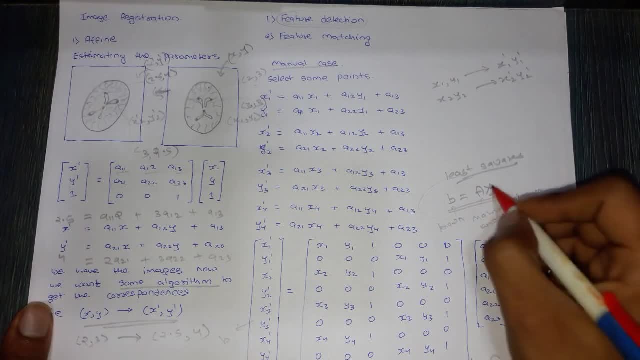 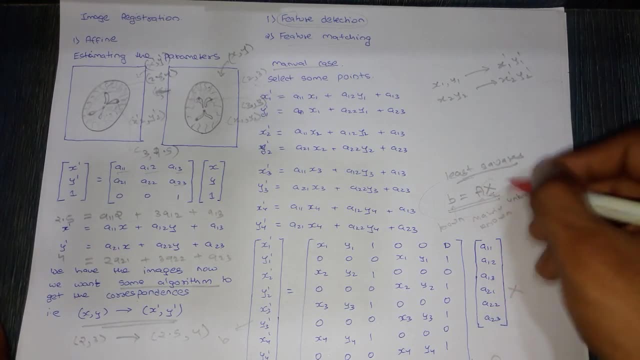 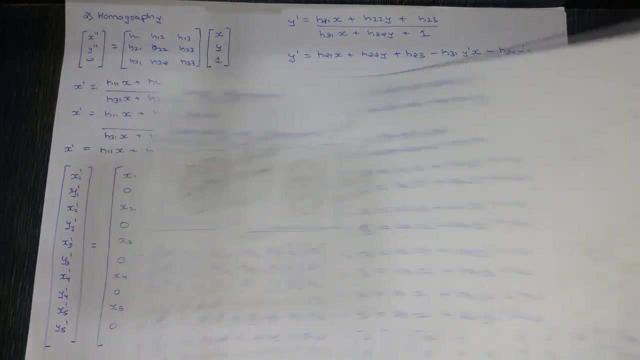 B is equal to AX. You can use least squares to know what is capital X. So we will discuss the least square algorithm in my next video. So we will see how can we find out this X. So that was for affine. Now let us see for homography. 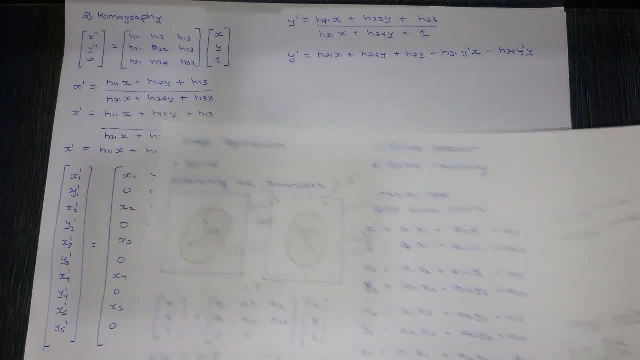 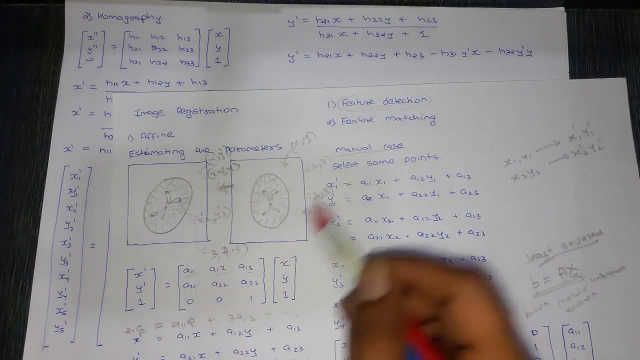 So affine is like a special case where you don't have these things, But in homography you have these things also. So the algorithm remains same. You will select some points And then you will have to do the least square. So just let us see how to get it. 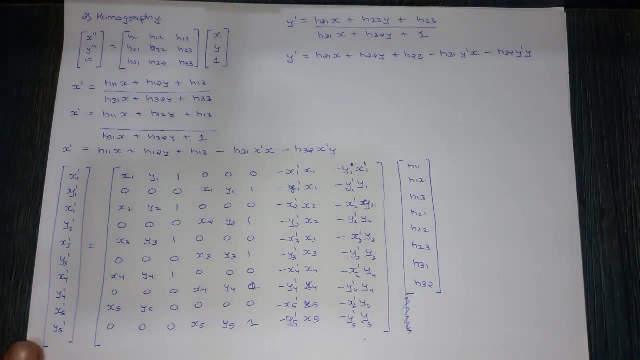 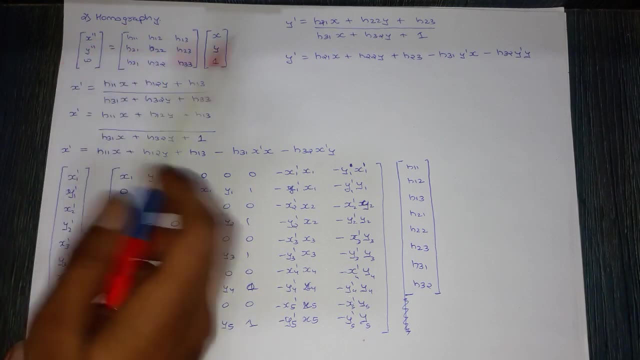 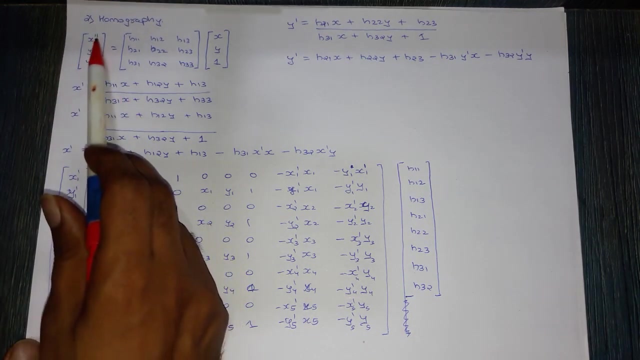 You will get this particular form of B is equal to AX. That's it. So this is the homography equations that we have. So we have this: X double dash is equal to H one one. this And then actual X dash is nothing but X double dash upon W. 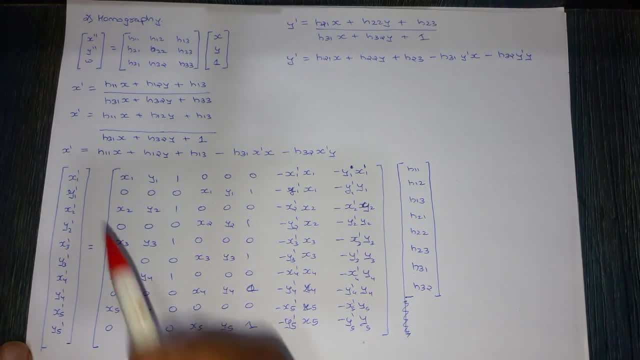 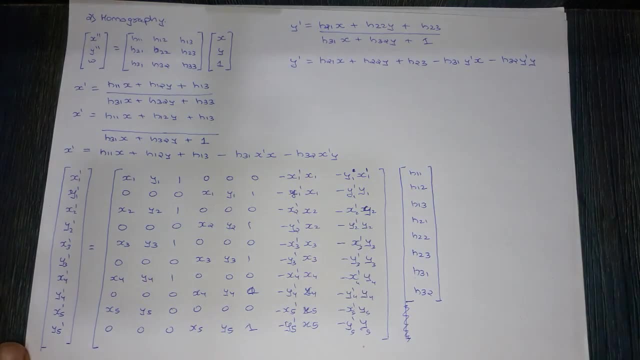 This is what we have seen in homography equation: Homography video. If suppose you have not seen homography, You can click this link over here And you will go to my homography video. So this is what we have Now, what we do now. 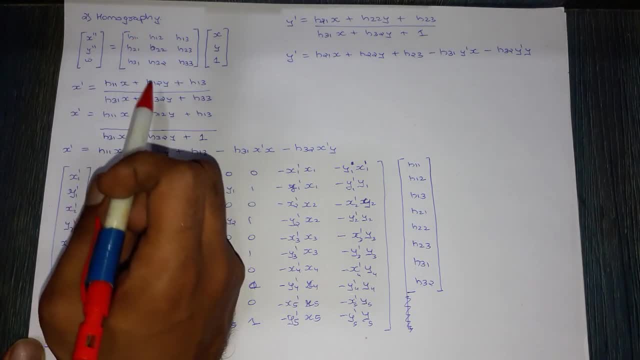 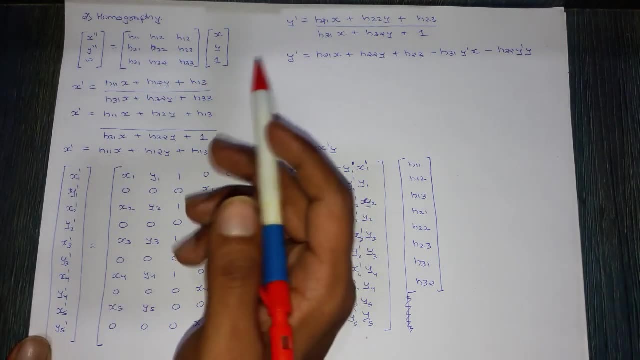 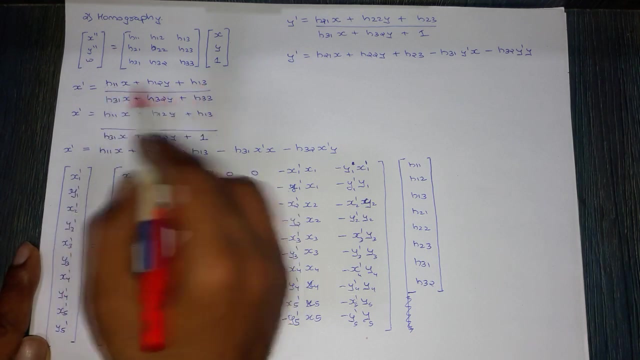 We have. if you see, we have nine parameters over here. So we can, by using a trick, we can reduce this nine parameters to eight parameters. So, simply, you have this particular equation for X dash. Now what am I doing is I am dividing this equation by H, three, three. 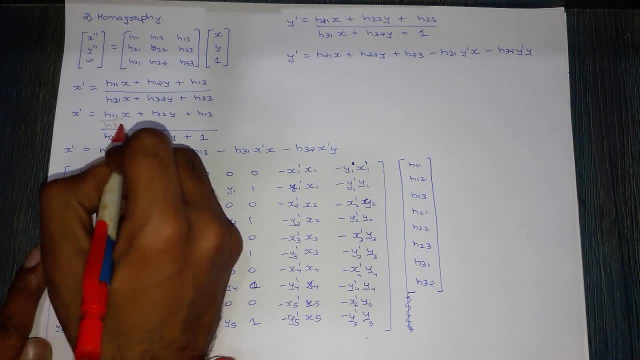 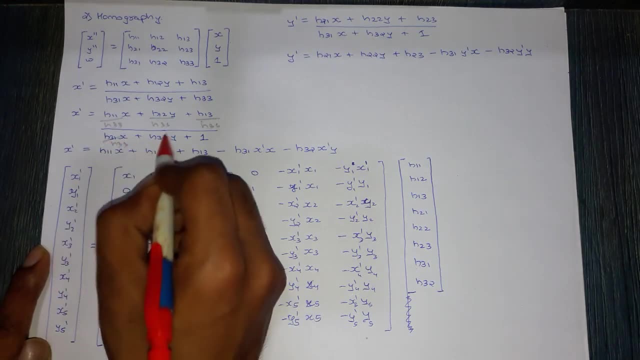 So let us see what happens. So this, divided by H three, three, divided by H three, three, divided by H three, three. So here there will be divided by H three, three divided by H three three. And here there was H three, three divided by H three three. 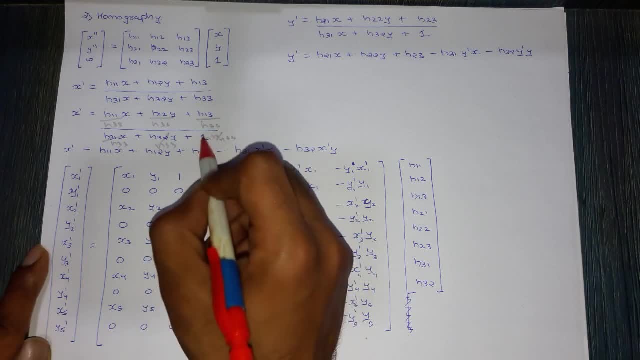 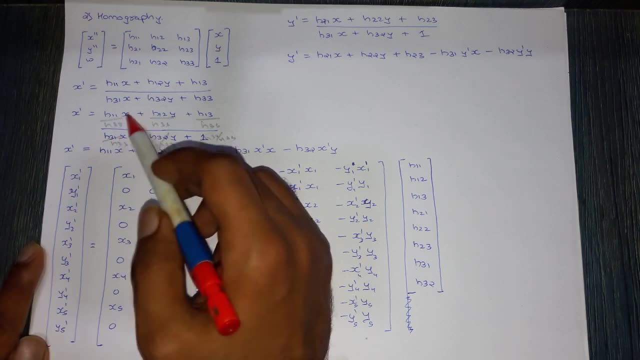 So what happens is: here you get a one, Here you get a one, And these things are anyways parameters. So H one one was a parameter. If I divide H one one with H three, three, that again remains a parameter. So I can find out H one one. or I can find out H one one by H three, three. 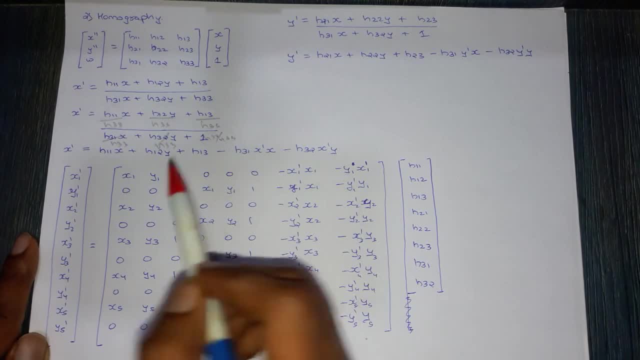 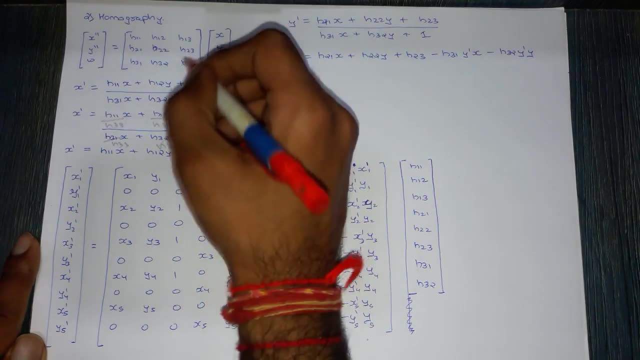 That does not matter Similarly for others. So by using this trick, what I have done is I have reduced this parameter. So now I don't need to find out this, I am just having a one over here, So please understand this thing. 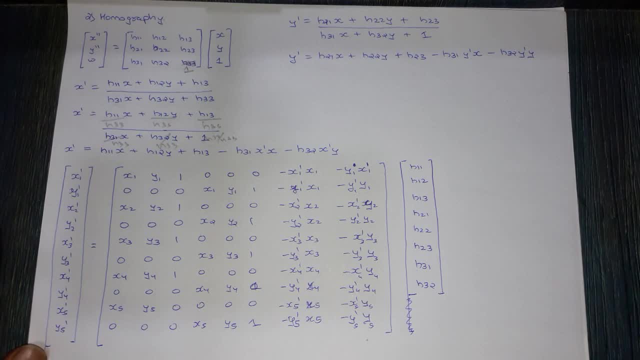 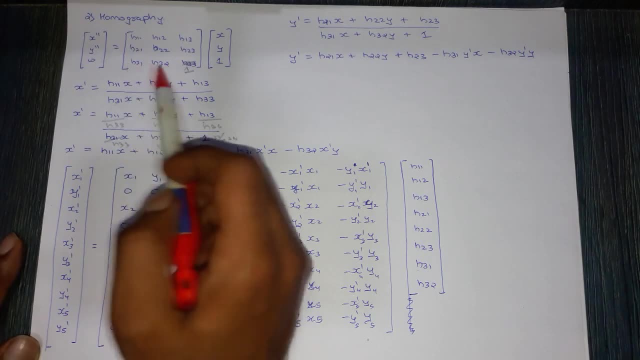 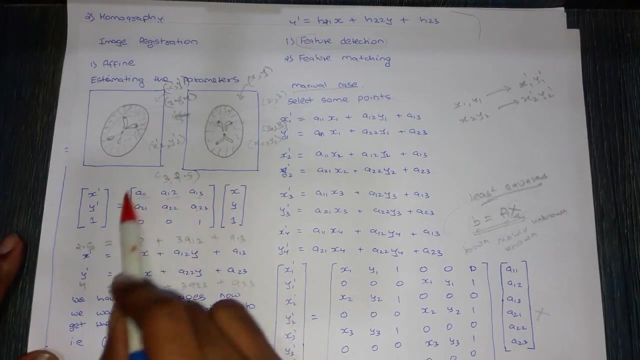 It is just to reduce the- what we say- parameters so that I can more efficiently calculate. So here, if you can see that I have eight parameters to calculate. Also one more thing: I forgot to mention that, since we had six parameters, So at least six equations we need. 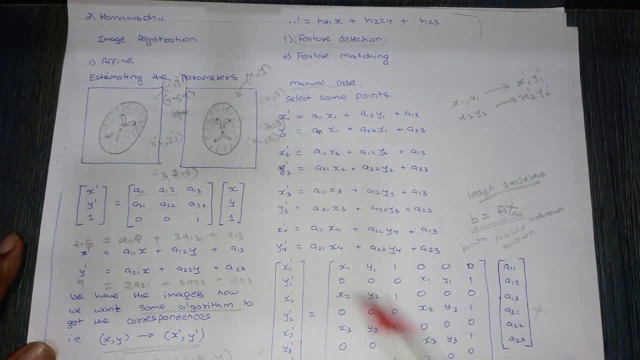 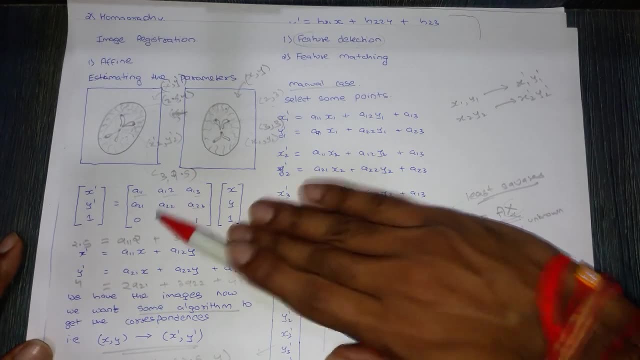 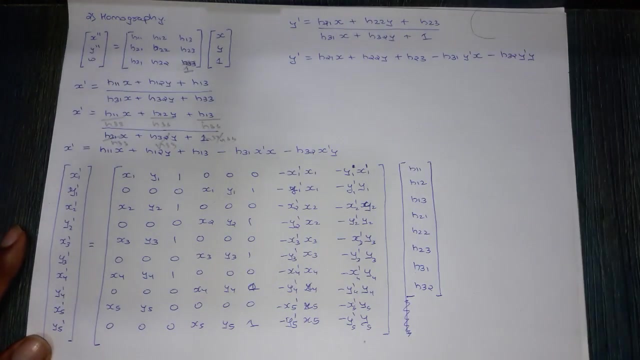 So here I choose four points, so that I have eight equations, which is okay, But you cannot choose two points. So if you choose only two points, you will only have four equations. Using four equations, you cannot solve six parameters. So that is also one more thing that you will have to know. 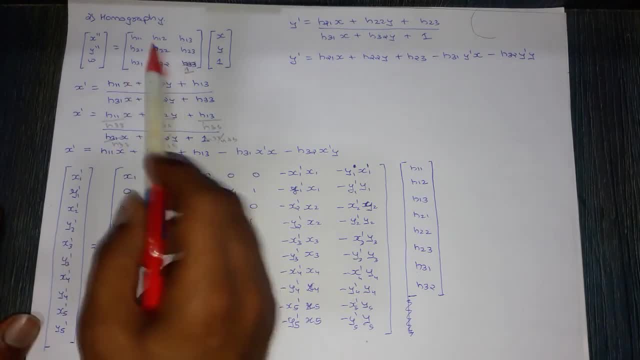 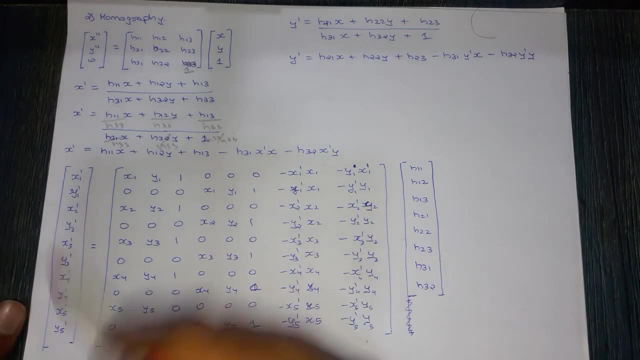 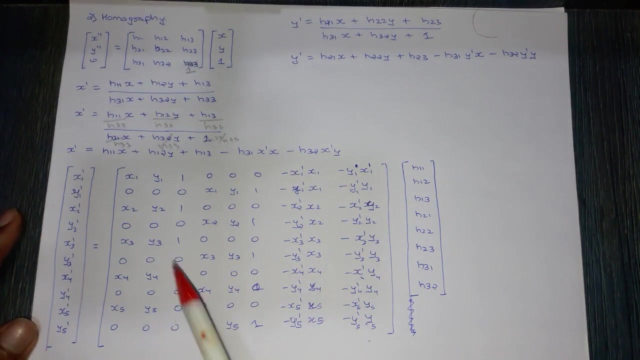 So here, since I have eight parameters, I need more eight or more than eight parameters. So we will see in least squares how we actually solve this thing, Or how do we solve with more equations and those sort of stuffs. So now we have this particular form. 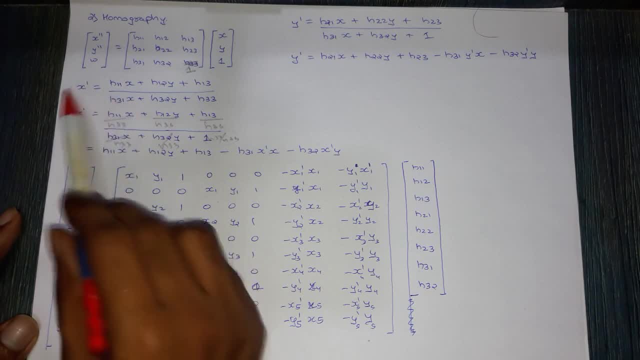 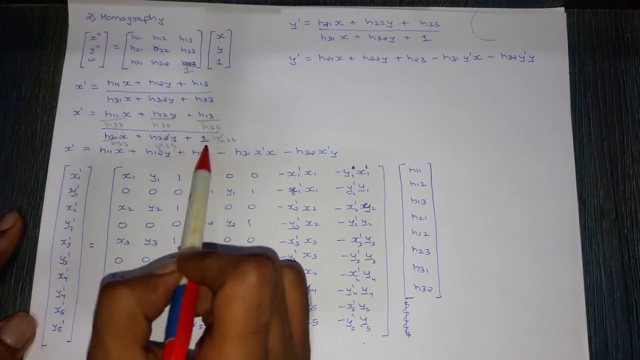 Now what we do is I multiply this denominator over here, So the denominator is multiplied over here. So what will I get is X dash into X into H three, one Plus X dash into Y into H three, two Plus X dash. That is what you will get. 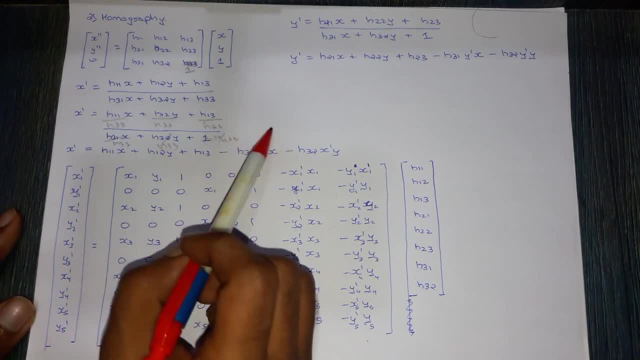 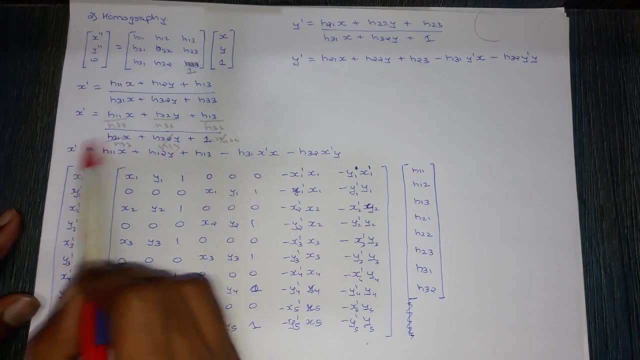 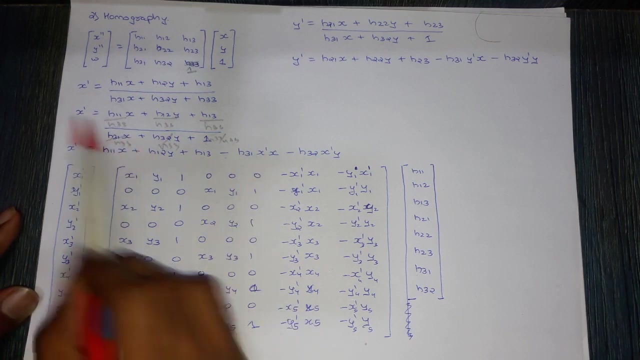 And then I take all those in the right side. So I will get H one, one X plus H one, two Y plus H three, one Minus. I will have one term: H three, one X into X dash. That will come over here. So minus H three, one X into X dash. 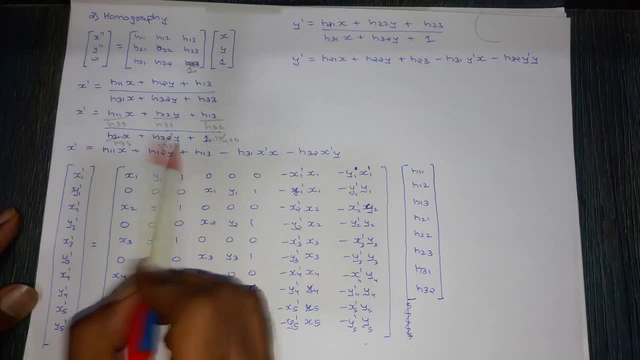 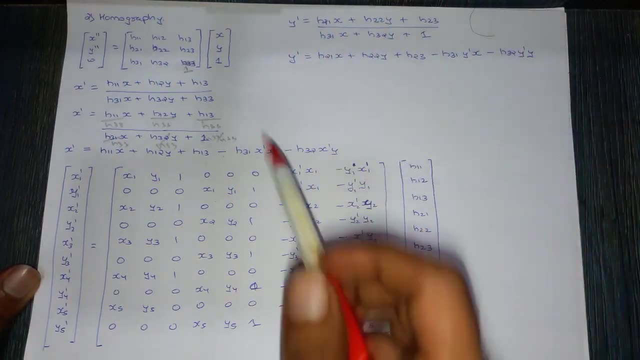 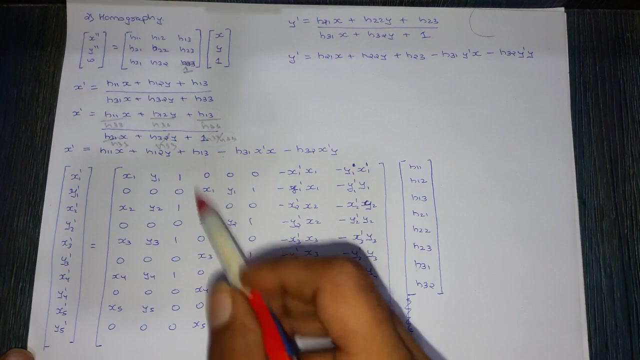 Minus H three, two H three, two Y into X dash. So that is what I will have. Similarly, I can do that for Y- Y dash. So the same thing I have done over here Now the same matrix I am going to form over here. 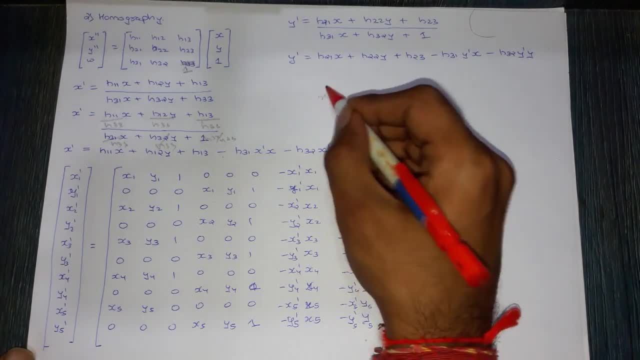 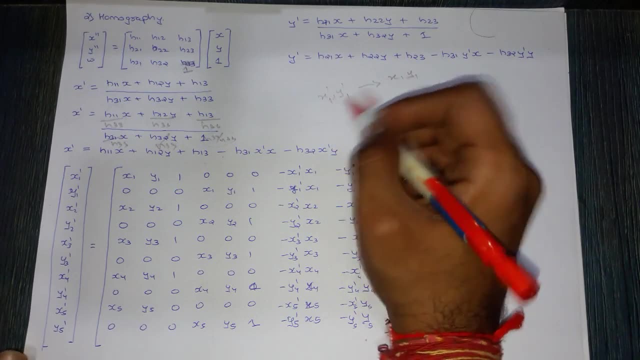 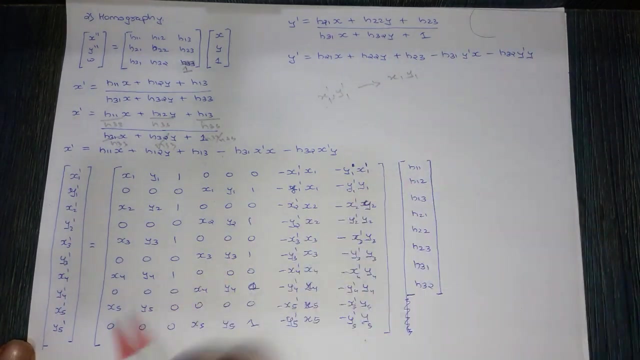 So you see that these are known. I have X dash, Y dash, So X one, Y, one corresponding. I have points X, one, Y, one corresponding to X, one dash, Y, one dash. So here I took five points, Because here I just have eight parameters. 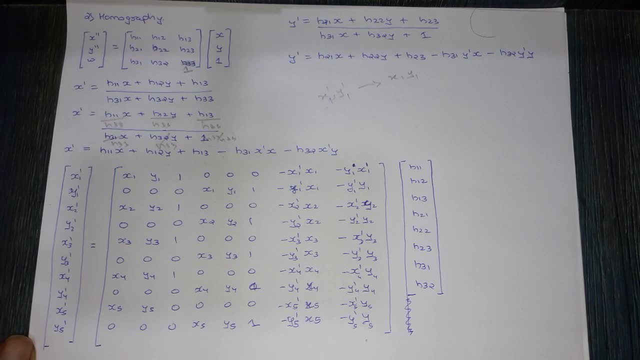 So I am taking a little more parameters So that I can have a better estimate, So that we will see in least squares how why this is good, Taking more parameters is good. So that is what we will see in the next video. So we have this. 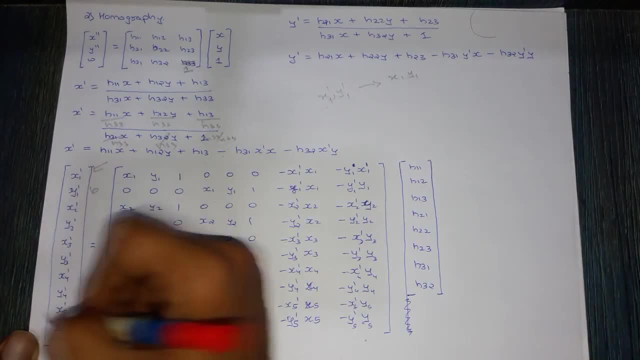 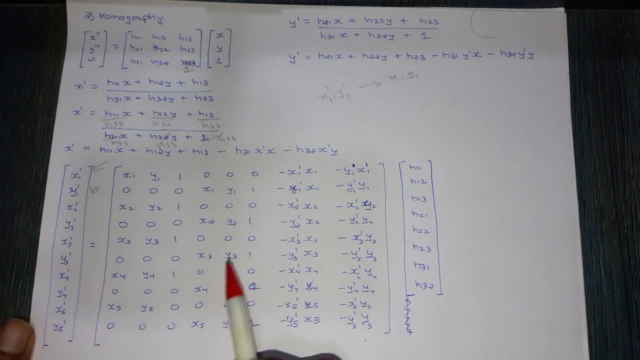 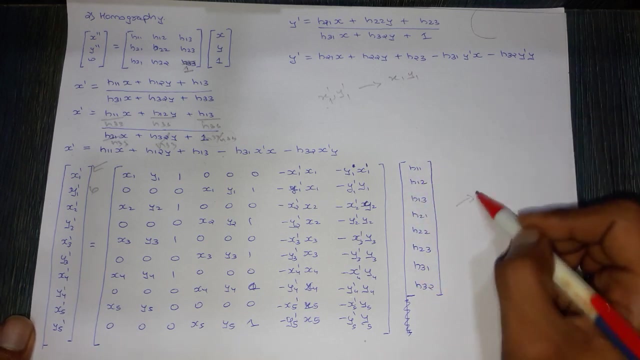 So this is known, So this becomes my B, which is known. I know X, one dash, Y one dash by those points selections over there And this particular thing we will see. how did we get this? And this is unknown. All my parameters are unknown. 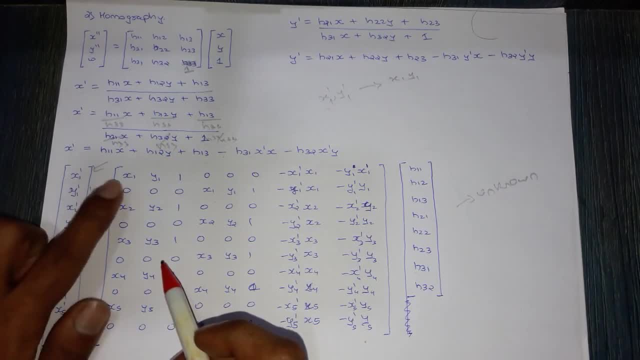 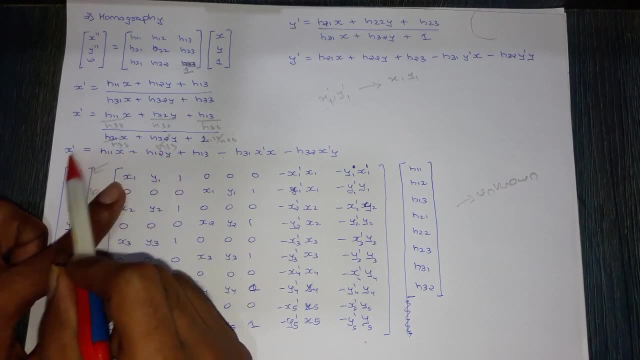 So now this thing, let's see how did we get So you see that there is X over here, So there will be X one, Y one, X two, Y two, X three, Y three, correspondingly: X one dash, X two dash, X three dash and the story. 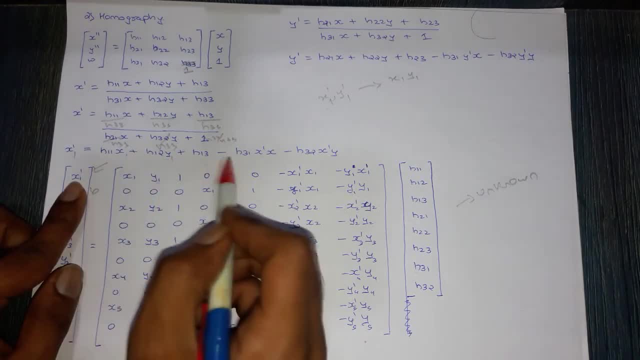 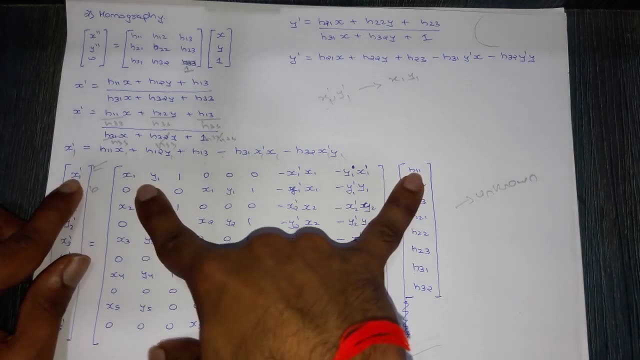 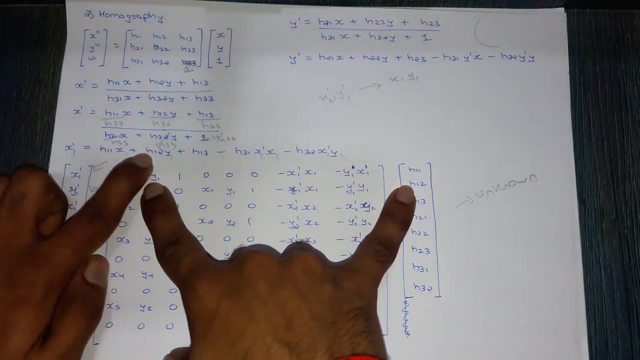 So for say, let me take first point case. So here, this is the first point case. So you see, X one, dash is nothing but X one one into H one, X X one into H one, one plus Y one into H one two plus H one three. 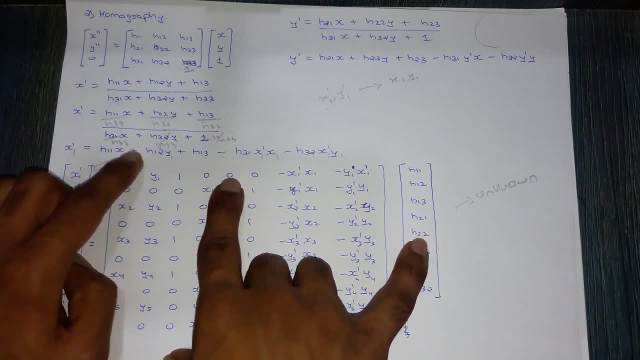 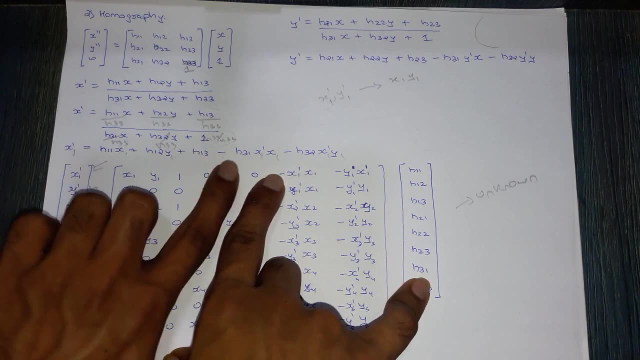 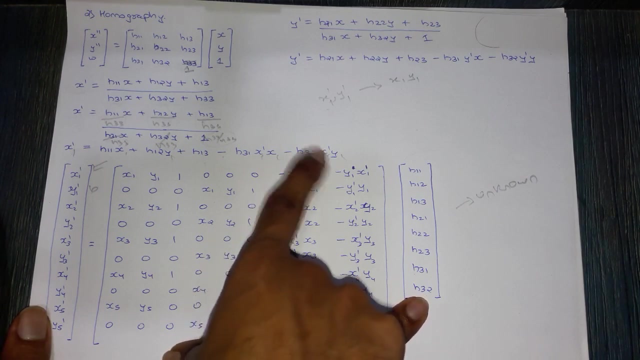 And I don't have H two one over here. I don't have H two two over here. I don't have H two three over here. Then there is minus H three one. So minus H three one into X one, dash X one. and minus H three two into X one, dash Y one.